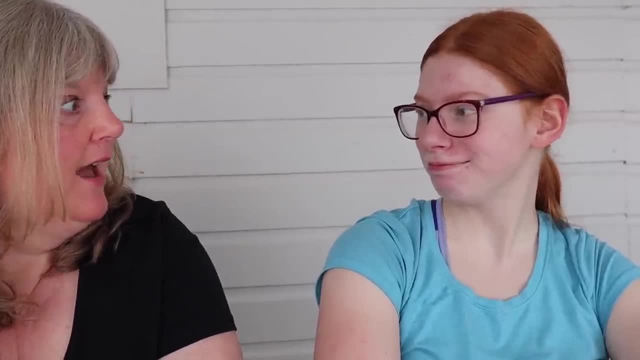 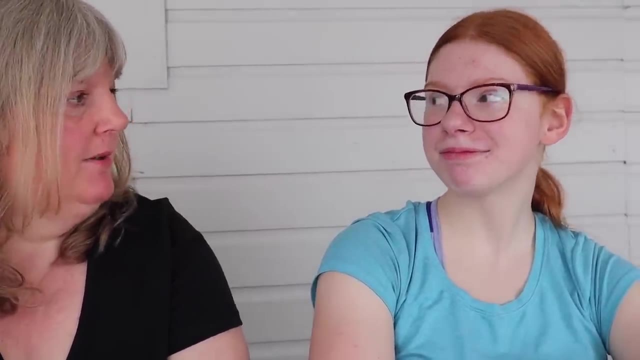 Welcome back. Today is cooking day. Yum, How did the shopping go? So shopping was a little bit harder than we thought it was going to be, wasn't it? Yes, Okay, but that's why we're doing all this. We're doing all of this to learn our skills. Yes, 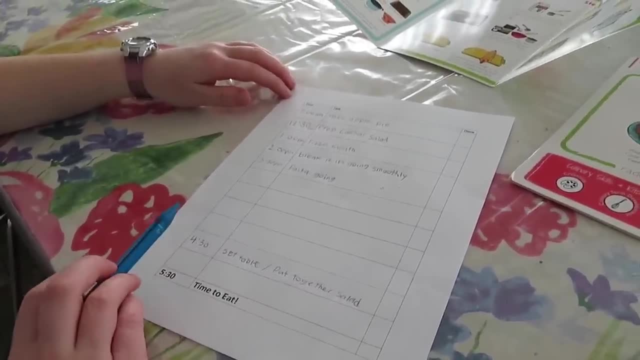 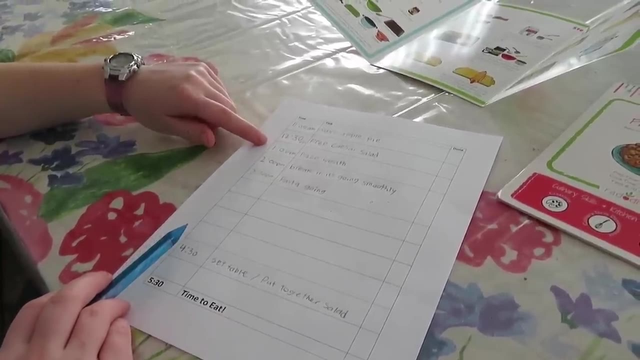 So you've got a plan here: Yeah, You're going to make your apple pie. Yeah, From 11 until 12, 30. Mm-hmm. Then you're going to prep your Caesar salad- Yep, And then you're going to start making. 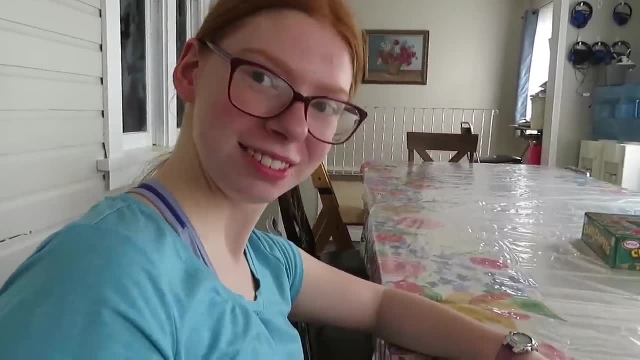 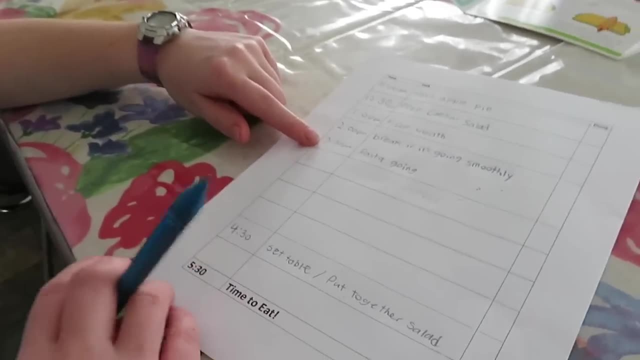 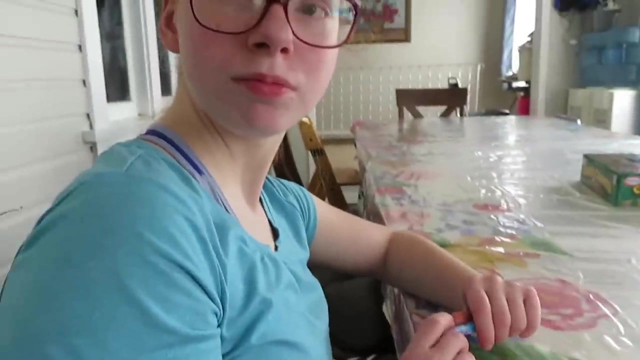 your pizza. Then you get a break. Yeah, Assuming everything's going smoothly. Yes, Then after your break, I'm going to get the pasta going. You're going to get your pasta going 4- 30.. I'm going to set table and put together salad. So are you going to set the table? No, I'm going to ask. 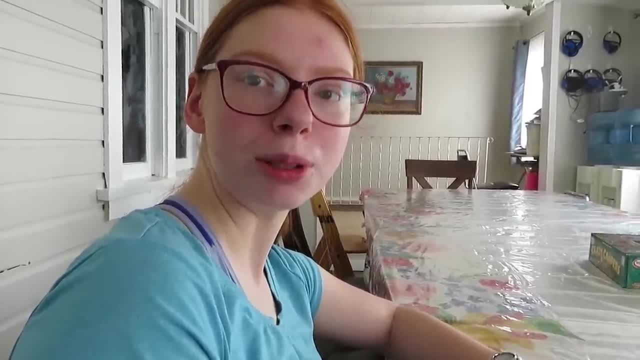 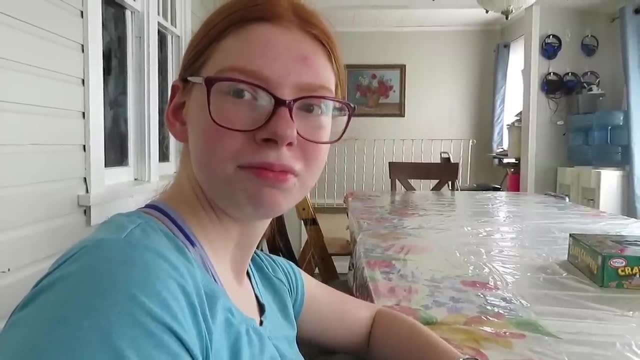 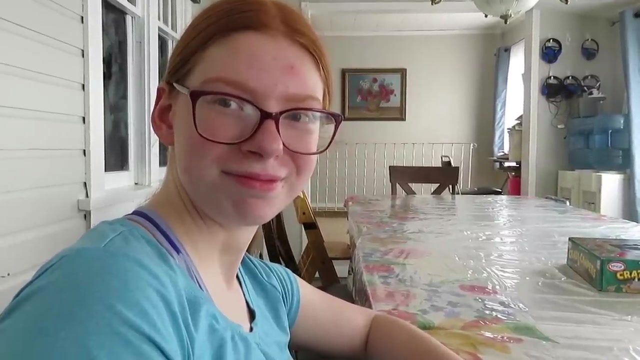 someone else, or probably two, to set the table, And all going well, everything's going to be coming together about five o'clock, Yep, Okay, And then the plan is to be completely ready by 5: 30. Do you think you can do this? I hope so. 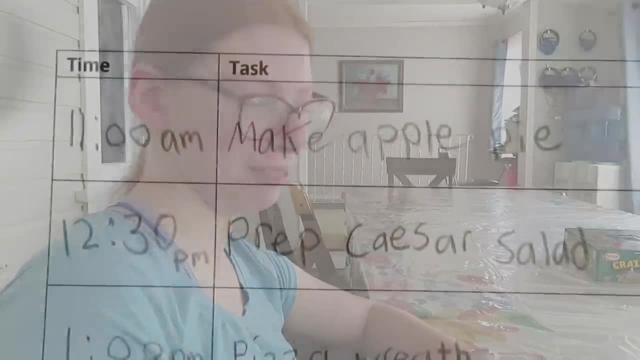 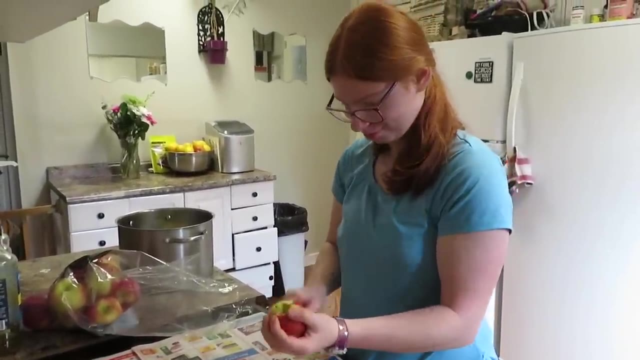 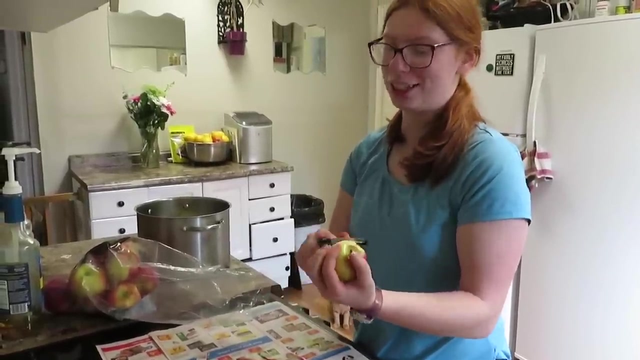 Are you ready to go and try? Yes, Okay, let's get going. Okay, So you're starting with the pie. Yeah, That's wonderful. What have you learned so far? That you don't need a special peeler for apples? I thought you did. 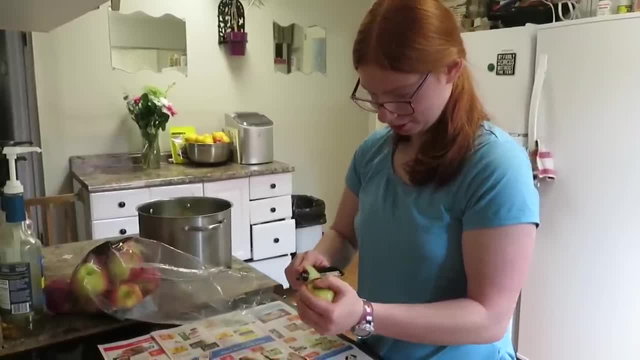 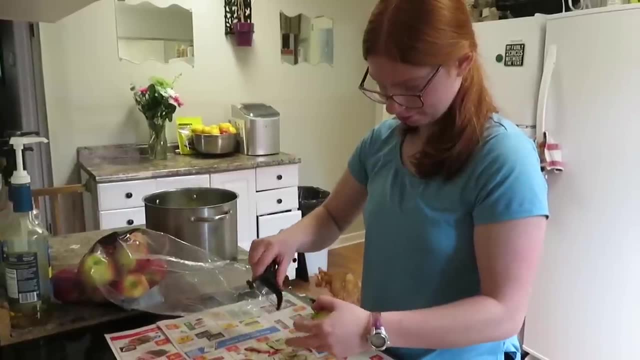 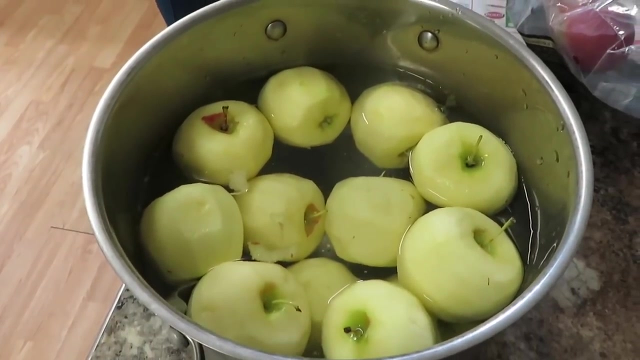 They use the same peeler as you do for other vegetables like potatoes. Yeah, And is it much different peeling an apple than it is a potato? No, not really. It's just easier to peel because it's not as thick. I could go bobbing for apples in this. I know That's what. 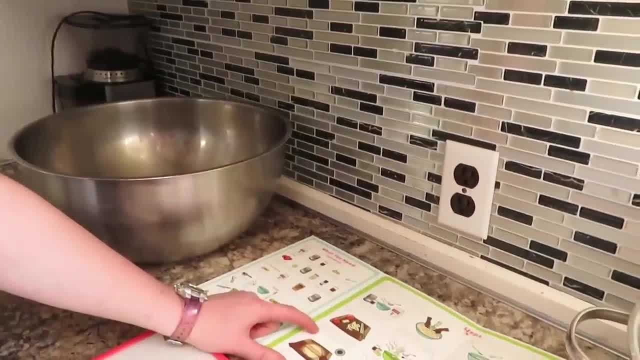 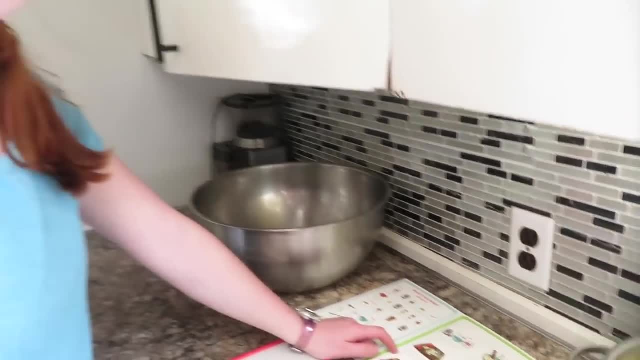 I was thinking as I'm peeling, Prepare filling. Peel apples- optional- Cut sideways away from the core, Then cut into pieces. Peel apples- optional- Cut sideways away from the core, Then cut into pieces. So do you know what that means? You've got your apples peeled, So what are they wanting? 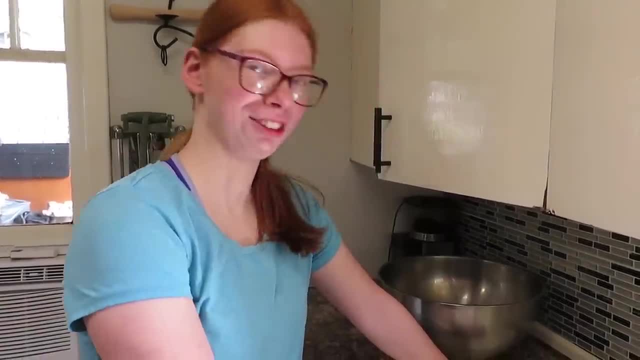 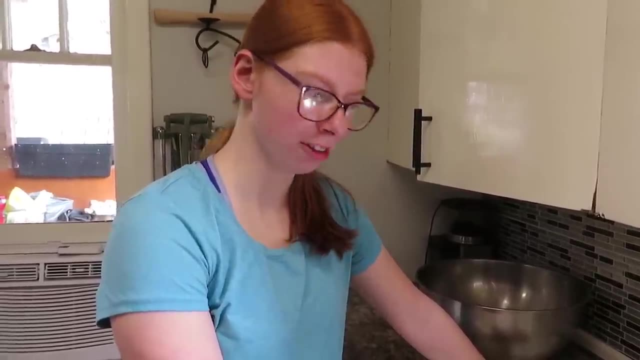 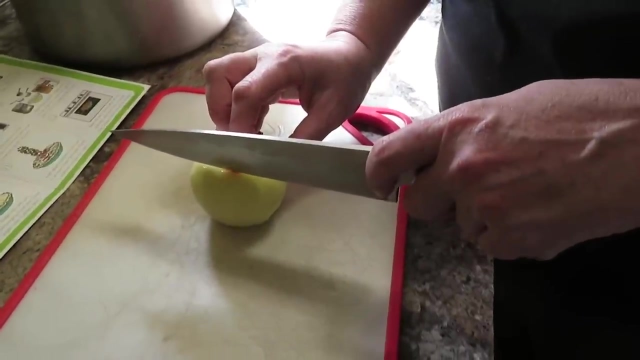 you to do? I'm not too sure. Okay, Well, you're going to cut up your apple. We're going to take the core out and we're going to slice it up. Okay, Do you want me to demonstrate and then you're going to do it after me? Yes, Okay, So we're going to cut down this side here, So see, 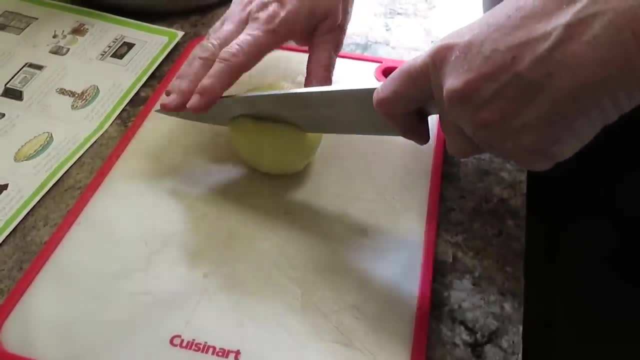 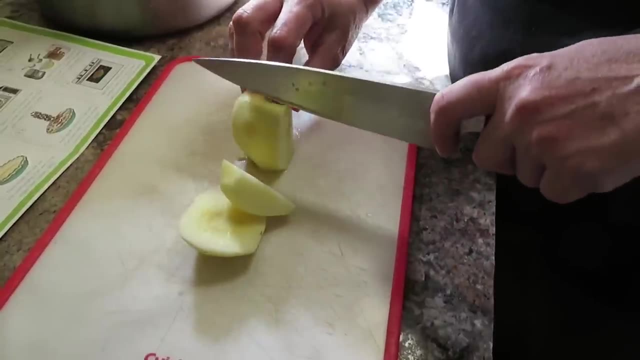 we want to cut, not on the core, So we cut down here, Then we're going to turn it, We're going to cut down here, We're going to turn it, We're going to cut down here, We're going to turn it, We're. 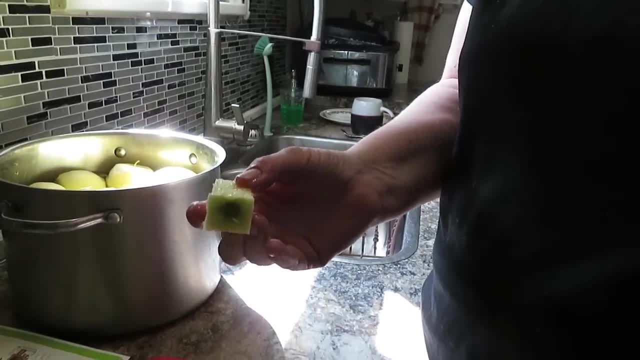 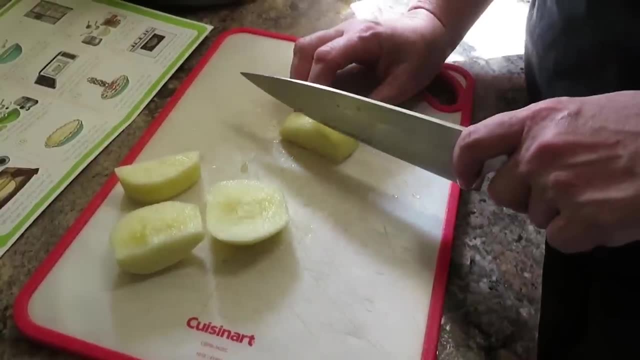 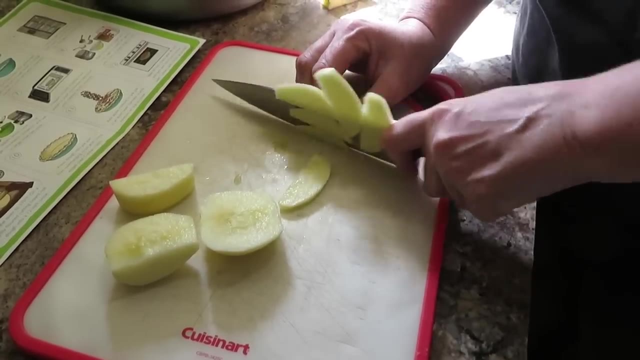 going to cut down here. This is the core, because we don't want the core in our pie. No, Okay, Okay, I'm not done. Now we have our four chunks. We're going to cut little slivers Like that, Okay, Then we'll get the other pieces. 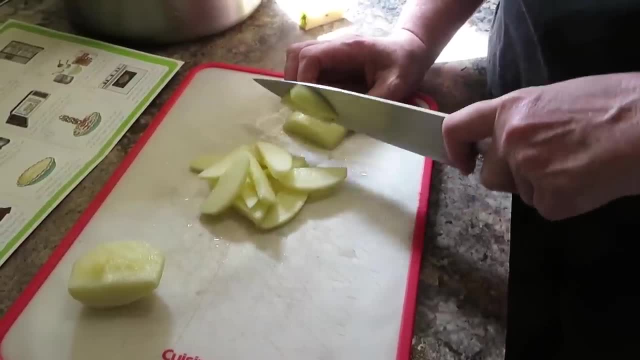 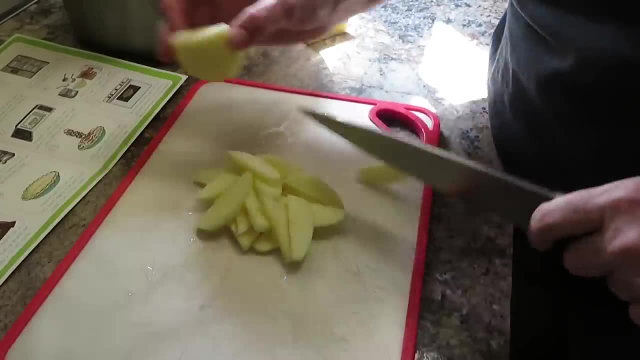 And by doing this way they're all similar shaped and similar sizes. Can you think of a reason we want them to be similar sizes? So there's not really big chunks that we have to slice up here in our pie and there's not little. 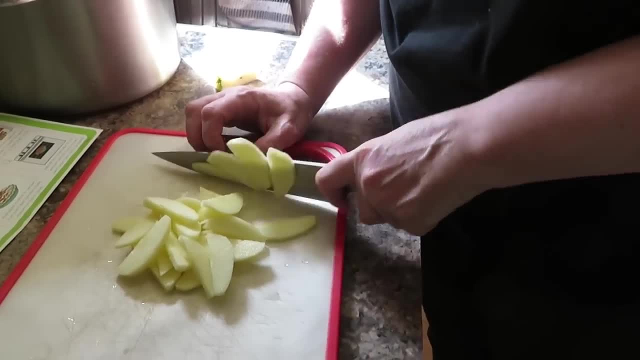 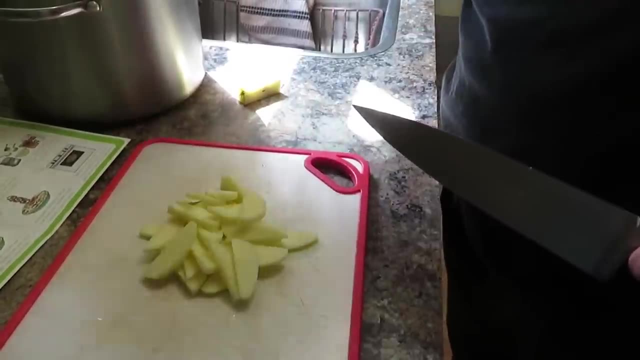 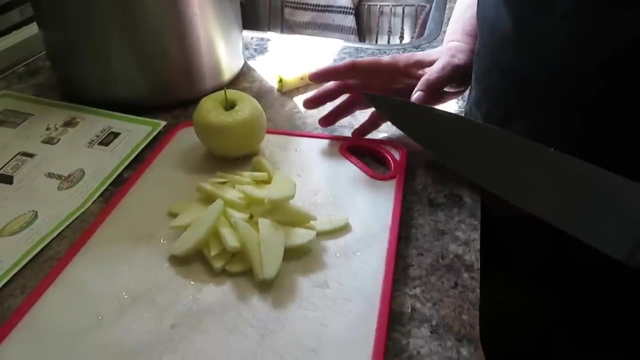 chunks to make it like Applesauce? I guess Yes, but also, we want it to cook at the same speed, Okay. So if I had an apple like this in my pie and then these slices, Okay, What's going to cook fastest? The slices, And then this part's not even going to be cooked, is it No? 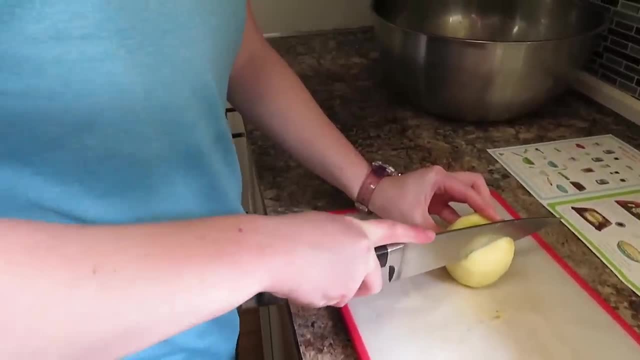 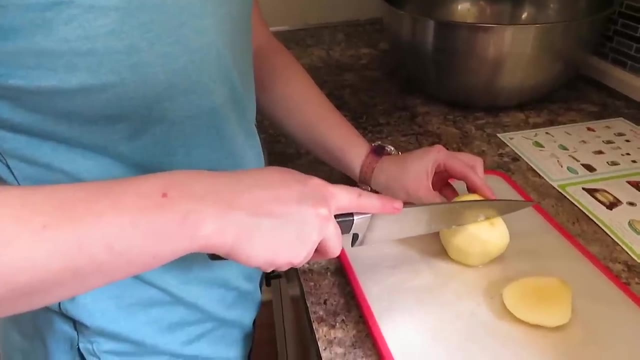 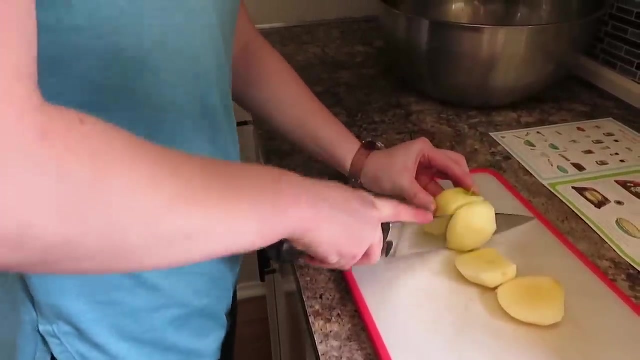 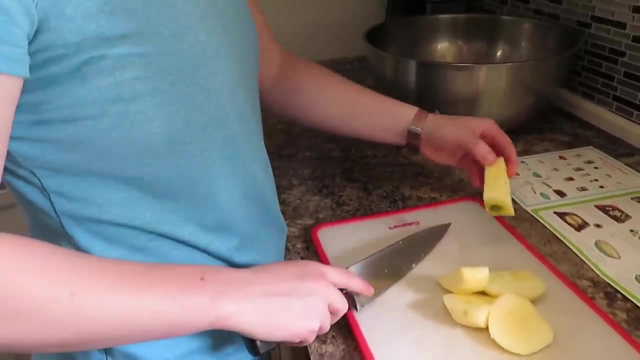 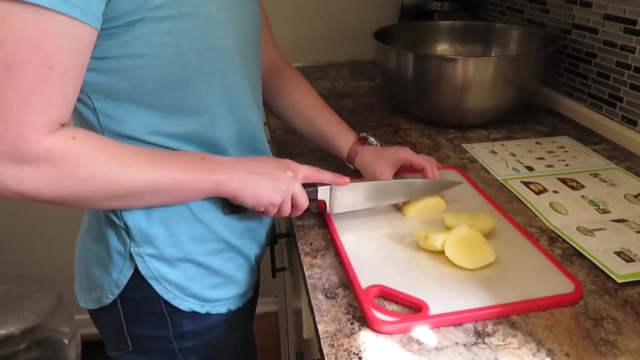 Yes, Next to the core You have to push hard. Then turn your apple Like this, Yes. Like that, Yes. Then your core can go into the compost, Okay. And then you cut them like this way: Yes, Okay. 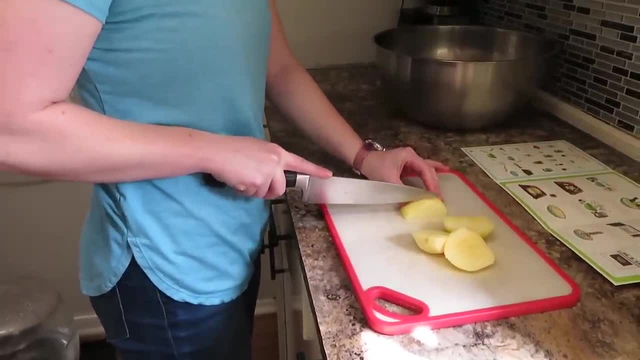 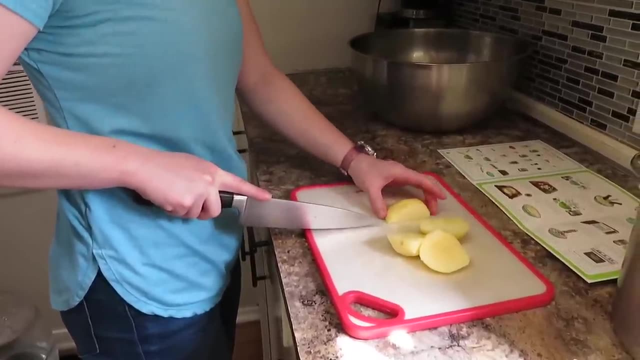 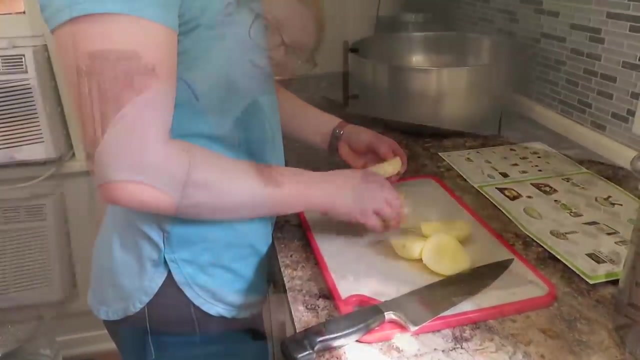 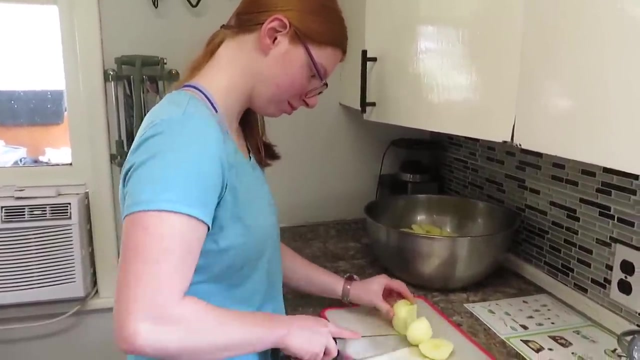 Okay, Okay, Okay, Okay, Okay, Is that okay, Okay, Is that okay? Do they look the same size as mine? Yes, Okay, then that's good. The last apple, That's good. So our apple cutting is taking a little bit longer than we had anticipated, isn't it? 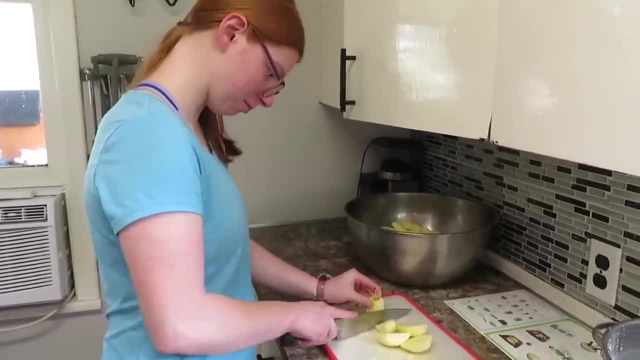 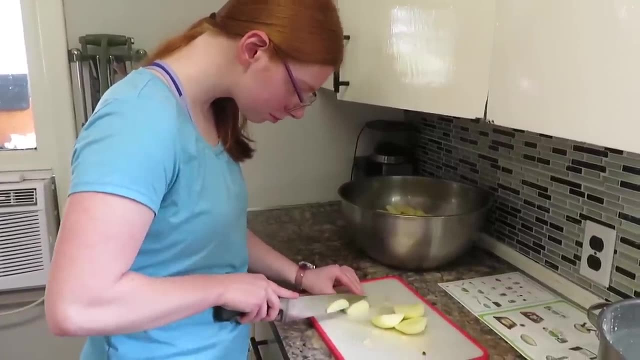 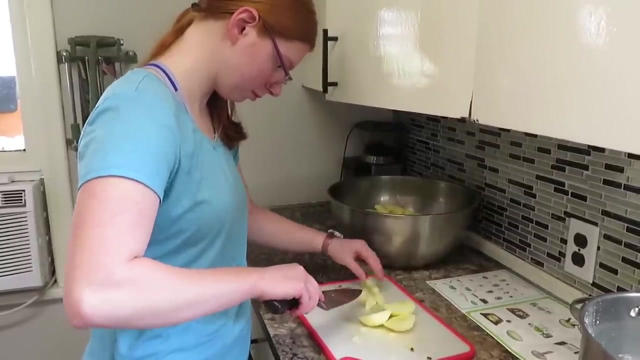 It's okay because safety first, Yes, But we've worked in a lot of leeway with your security, with your schedule, so you have plenty of time. right now we are at 12: 30, when we thought that the pies would be done and ready to go in the oven, but they're not quite ready, so that's okay. 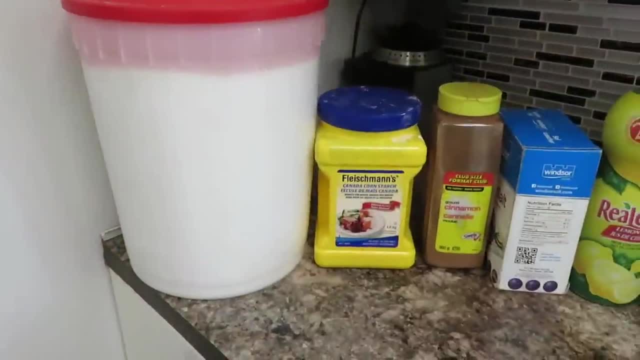 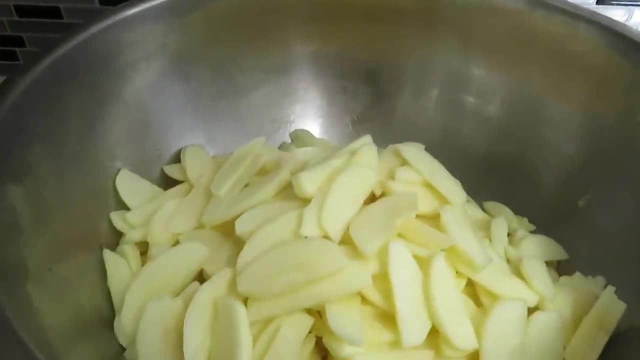 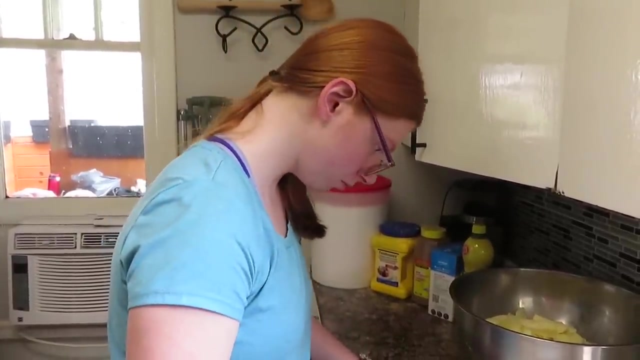 after your apples are sliced, what are you supposed to be doing with them? uh, stir apples, lemon juice, one-third cup sugar, cornstarch, cinnamon, salt and large bowl set aside. remember, you doubled the apples, so you have to double everything else. okay, so instead of one-third cup sugar, that'd be two. 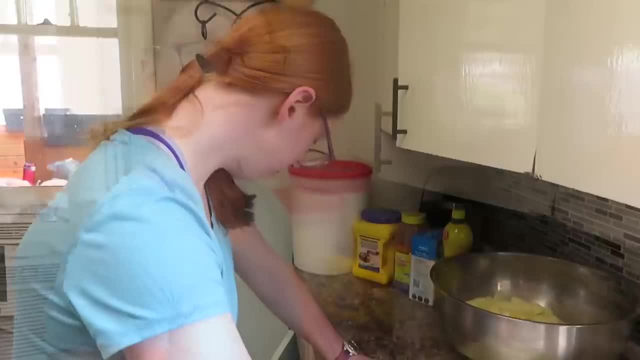 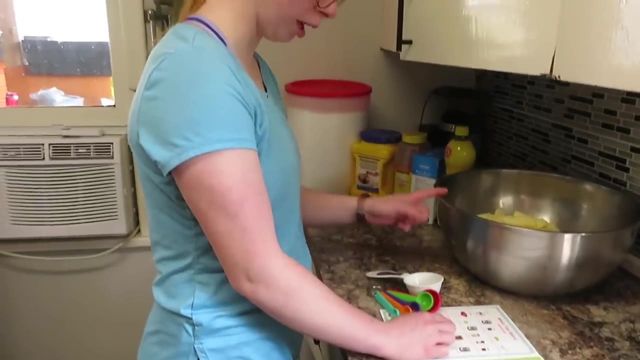 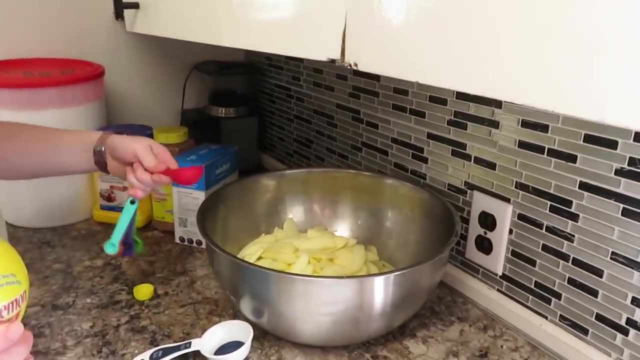 third cup sugar. right, correct, let's get it going. what does it say? after the apples, what's next? lemon juice. and we need one tablespoon of lemon juice. but since we doubled the apples, we need two tablespoons of lemon juice. okay, let me do this part over the sink. well, you can do it carefully over your apples. 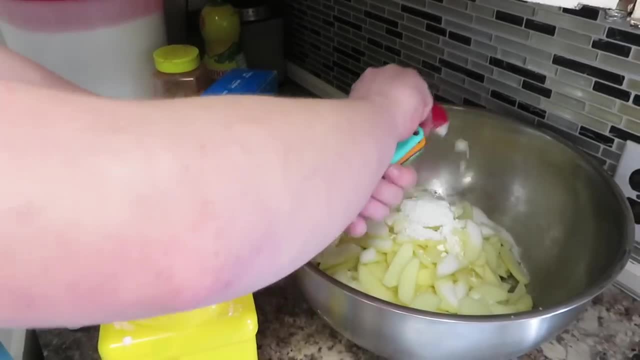 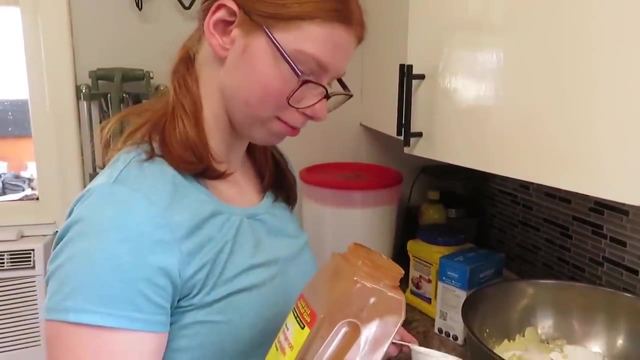 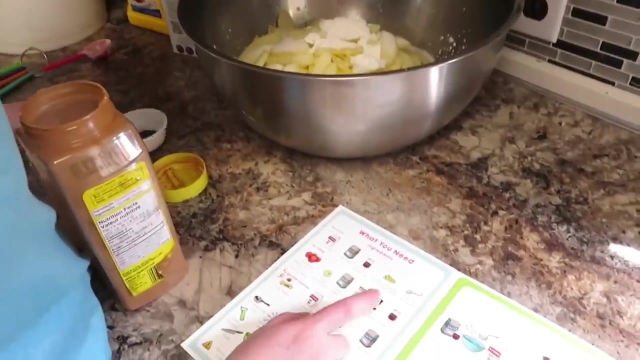 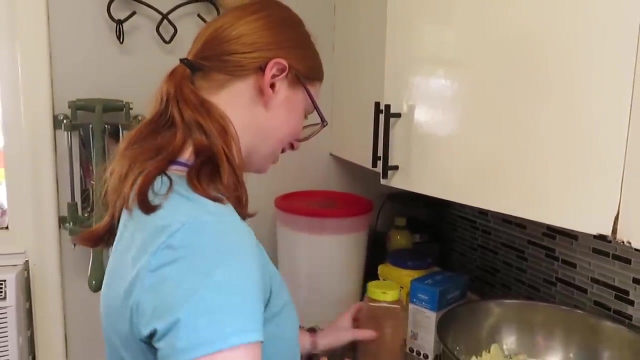 that looks good. okay, what are you doing? i'm gonna, pour carefully, pour your ground cinnamon into the one-third cup, and i need two of them, are you sure? oh, one teaspoon cinnamon. i was looking at brown sugar. you still need the cinnamon. yeah, why not? yes, so how much cinnamon are you gonna put in one teaspoon? 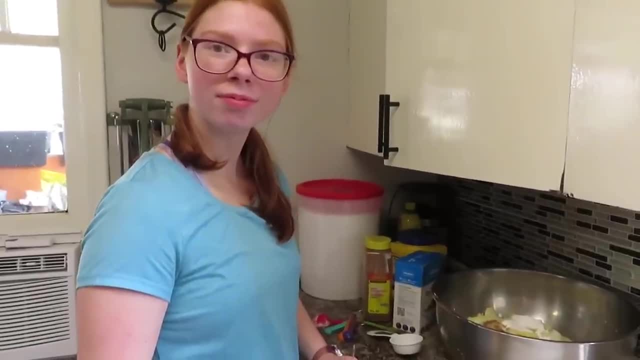 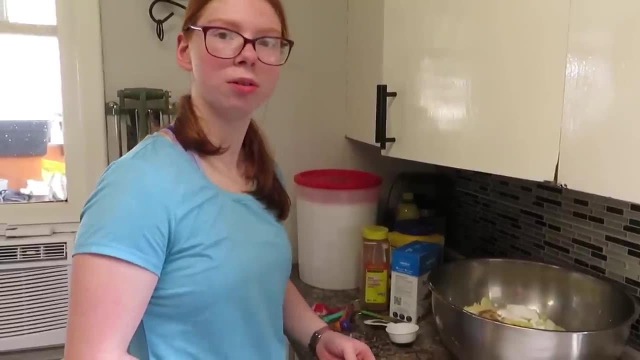 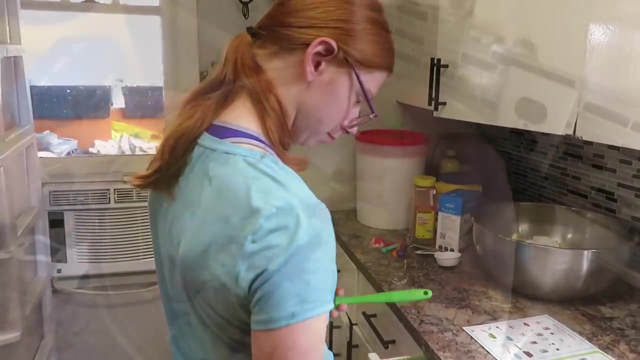 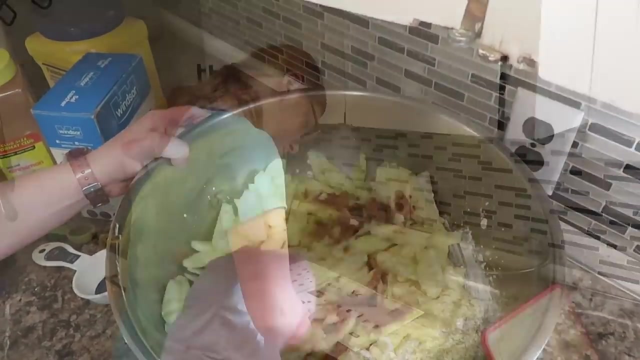 stir them all together? okay, stir them. you're gonna stir it carefully because you don't want to break up your apples. you just want them coated, okay, so get it. get a spoon or spatula and just be gentle when you do it. prepare crumb topping. heat butter in a small microwave safe bowl until melted. 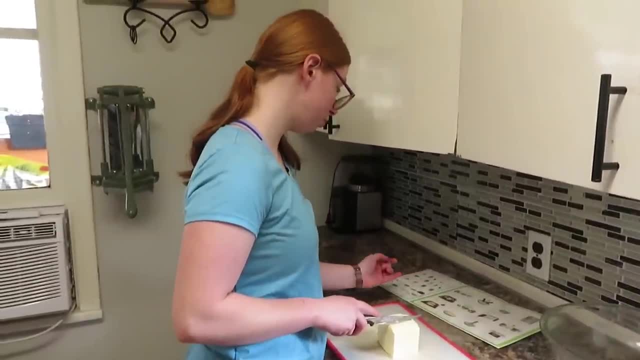 30 to 60 seconds. so it doesn't say how big the cubes need to be. so should i just do like. so it doesn't say how big the cubes need to be, so should i just do like. so it doesn't say how big the cubes need to be, so should i just do like. 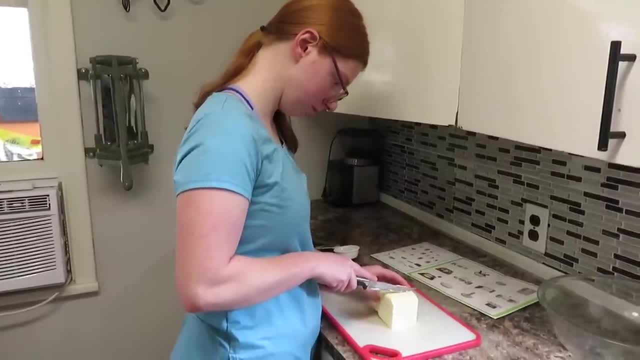 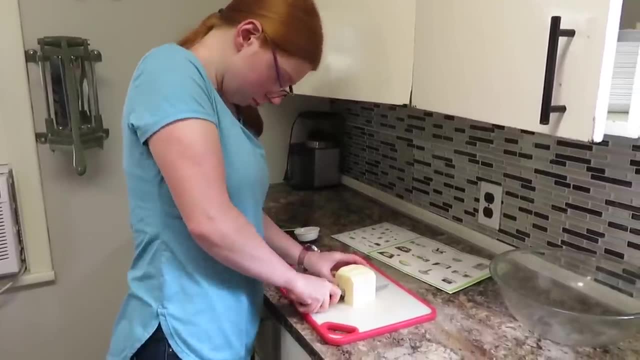 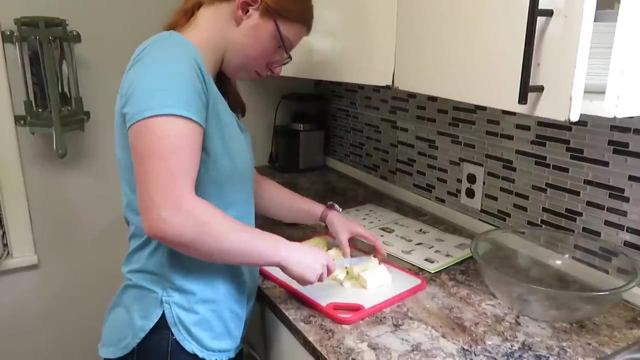 And just cut it up a little bit. It doesn't really matter the size, It's just to make it melt a little bit faster. So you could cut it into four, and that would be good enough. And then you can put it in this glass bowl, Because a glass bowl can go in the microwave, but a metal bowl cannot. 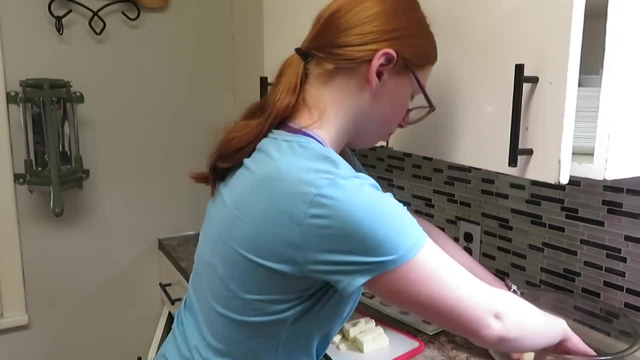 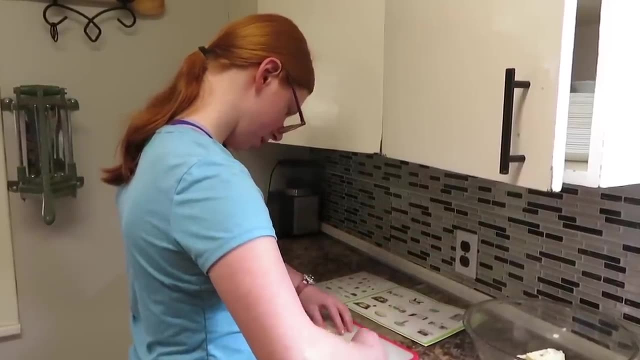 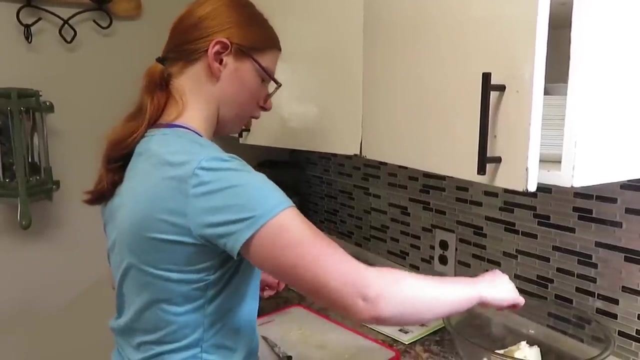 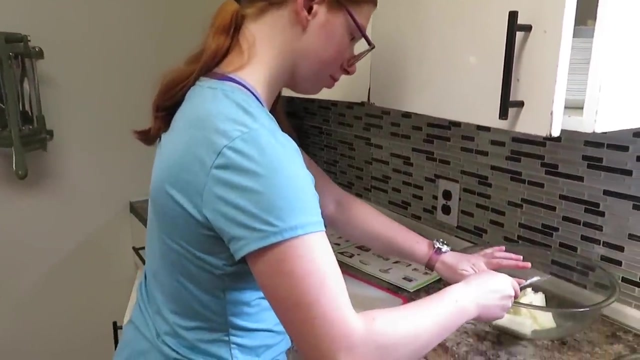 A metal bowl will start sparking and catch a fire and then our microwave won't work. So it's really important when it says a microwave safe bowl. I was thinking we could put it in one of our cereal bowls. We could, but it's asking you to melt this and then add some other ingredients. 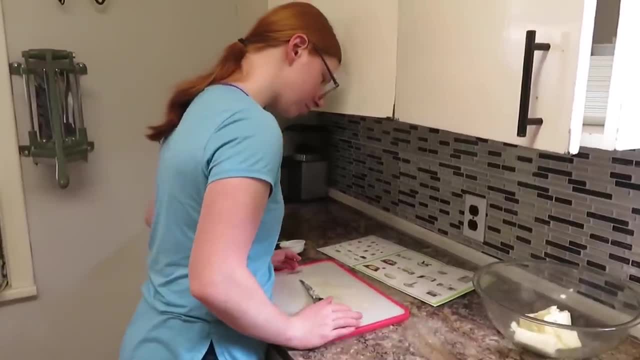 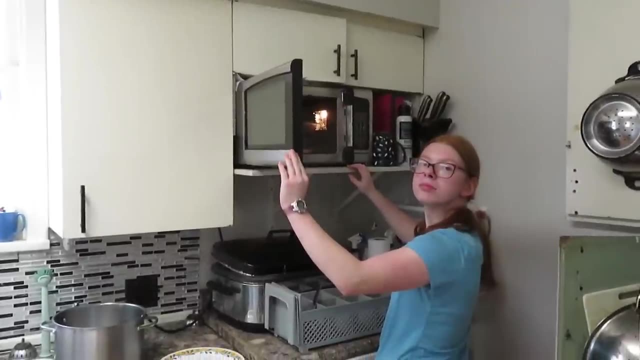 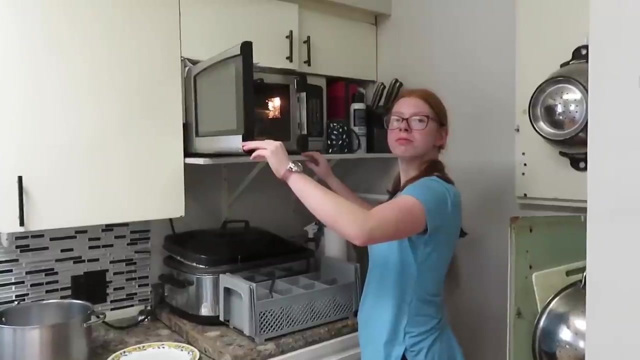 So if you use one bowl, that's going to hold everything, you're going to have less dishes to do. That butter is extremely hot, So if you pick it up and slosh the butter and it comes out at you, it's going to burn you. 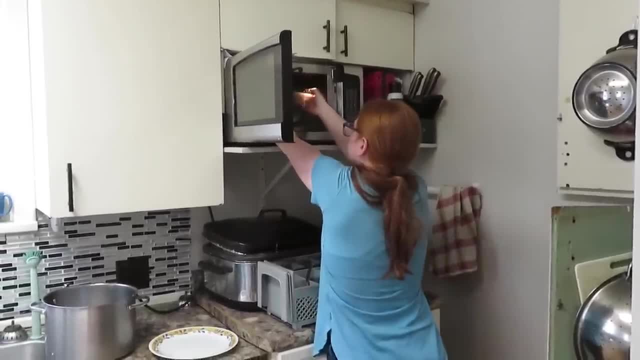 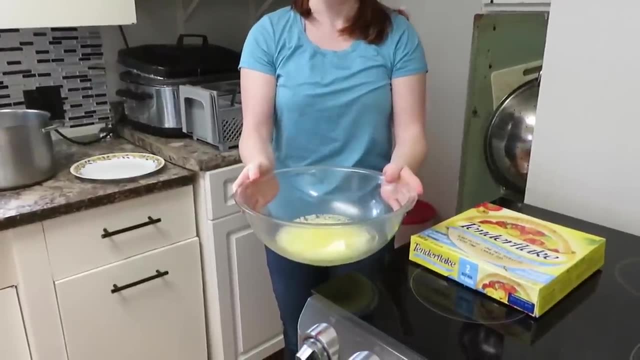 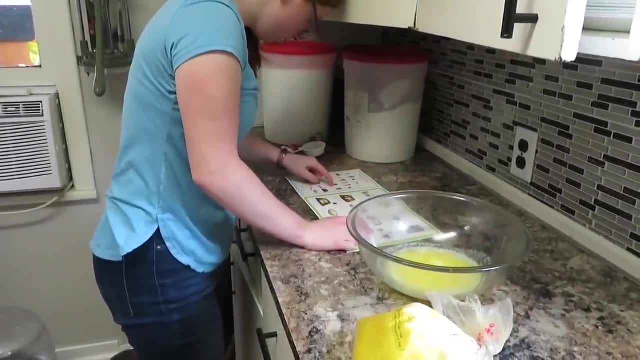 So hold it level and do it slowly. I think it'll be close enough by the time you mix everything together. I don't know how much flour- One teaspoon? Nope, that's not it. So look where it says crumb topping. 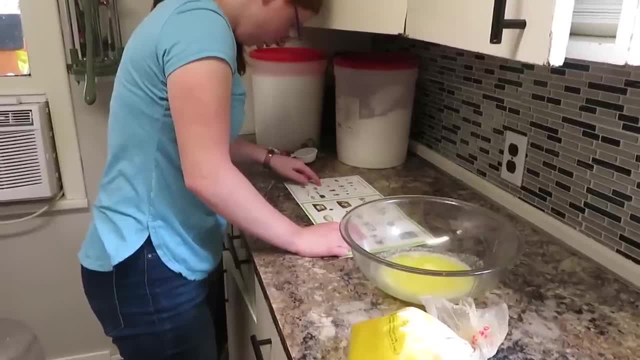 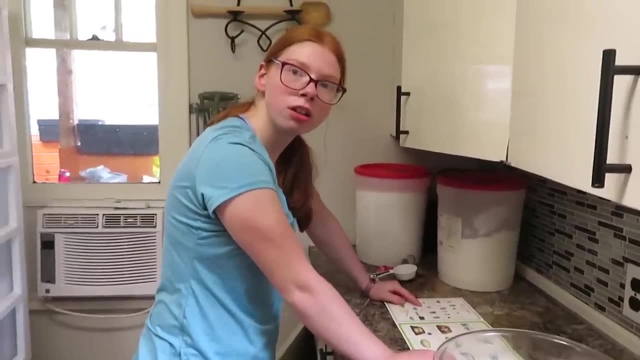 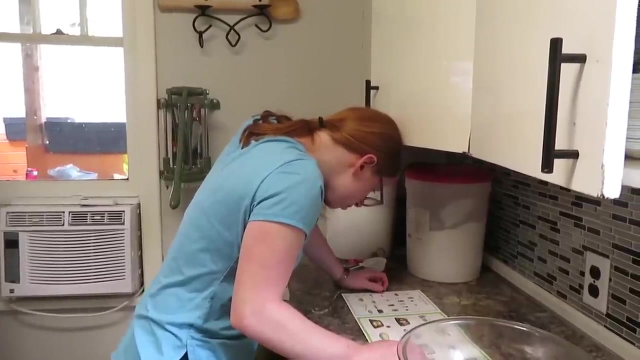 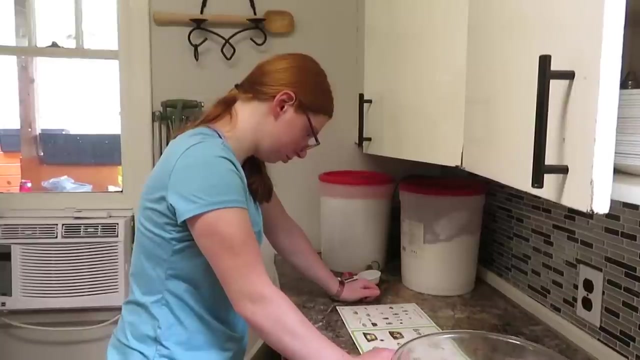 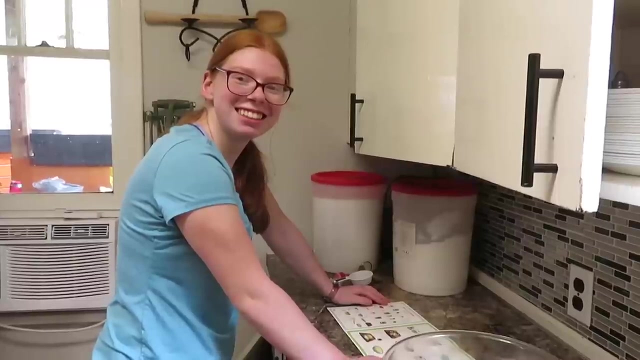 Yep, And follow that row. One and one-fourth cups flour, So that would be Two and one-fourths. Well, don't you have to double that one-quarter as well? So two and two-fourths. what does two-fourths equal? so two and a half cups, because a quarter plus a quarter equals a. 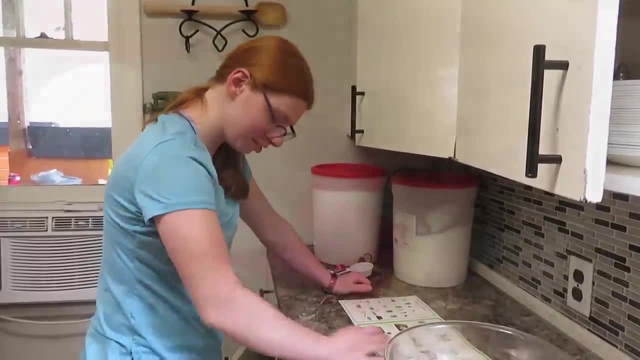 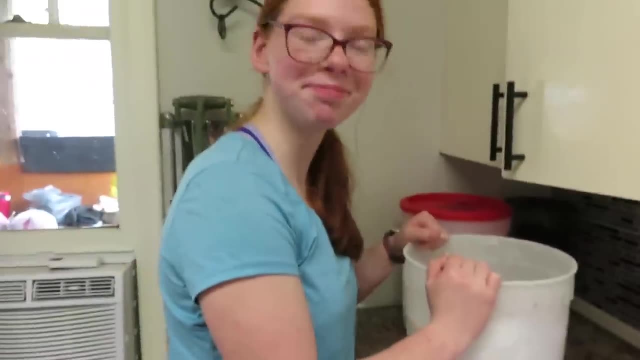 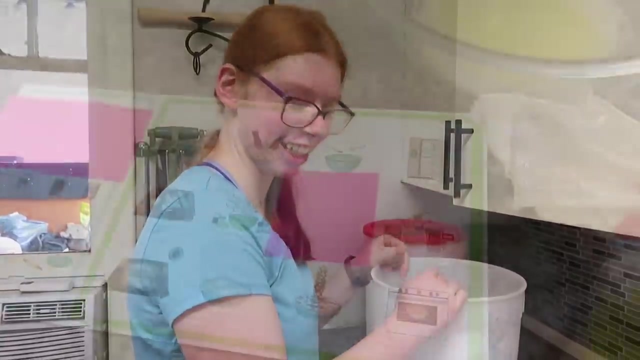 half. yes, okay, two and a half cups. so, because you're having trouble tracking, I put post-it notes to block out what you've already done. okay, okay. so those measurements you've already done. so this is what's left, to make it easier for you to track. also, put one here on the one that you've. 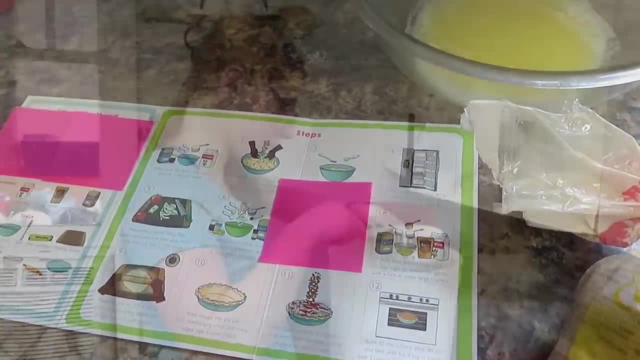 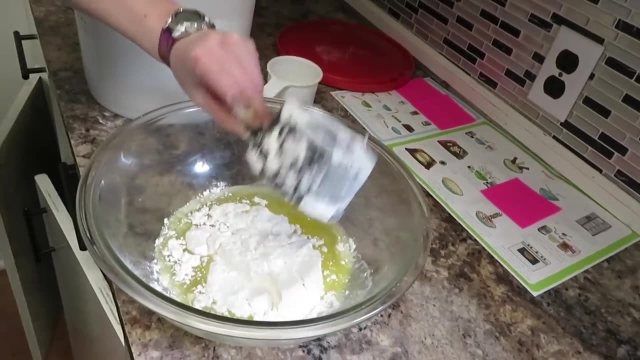 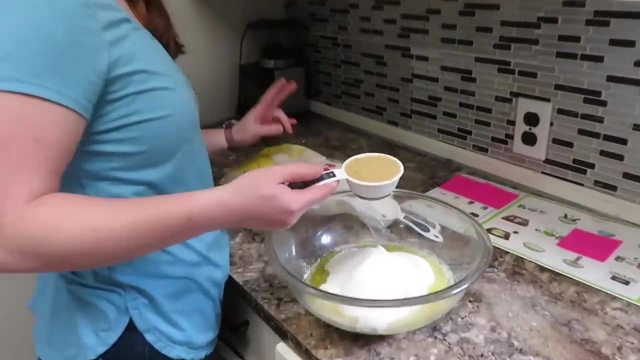 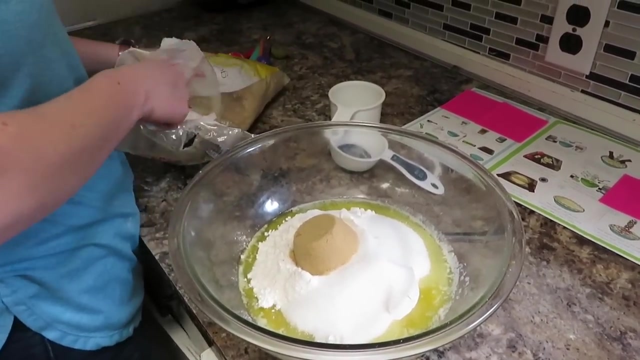 just done so, then you can move it over as you go. okay, one, I said two and a half, it's next brown sugar. two one-third cups- okay. one thing I like about brown sugar: it kind of like forms like snowballs or something. now, what do you need to do with? 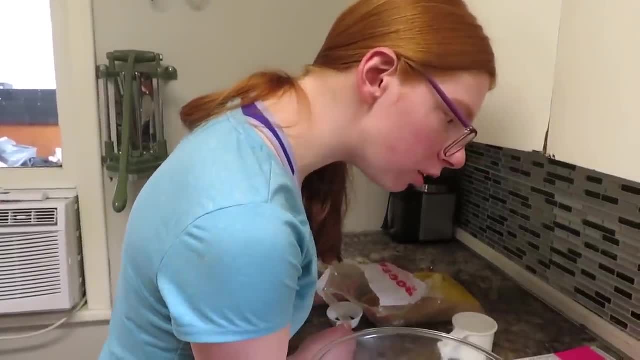 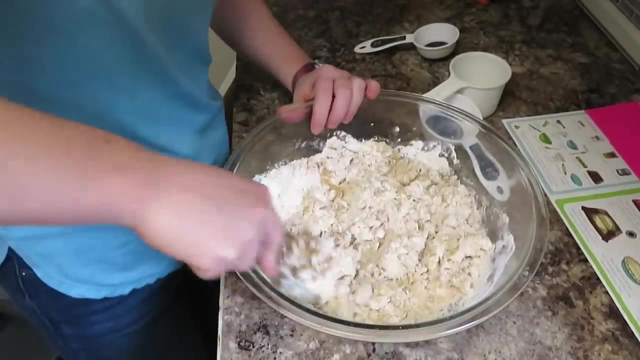 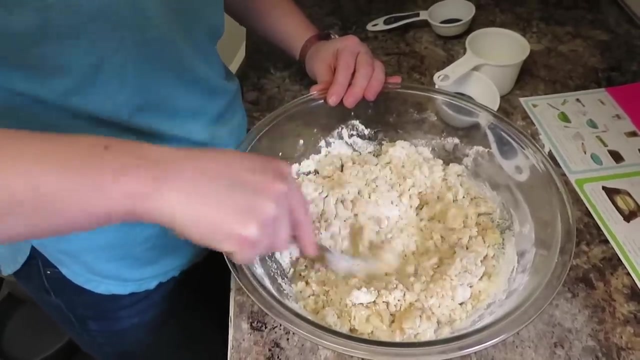 this: stir gently with a fork to make large crumbs. this has been easier with the like a mix or something, but you don't want it smooth, you want the crumbs in there, because it's your crumble type topping. so I moved your post-it notes. mm-hmm, what's the next step you need to do? 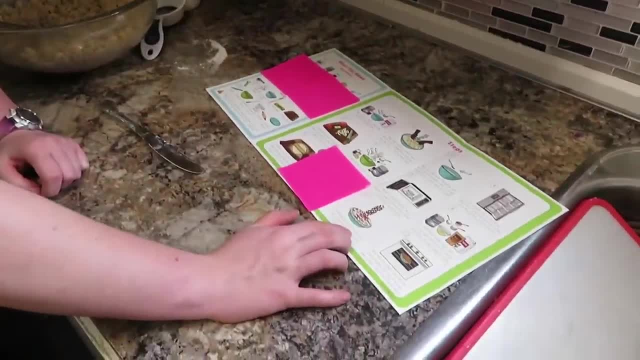 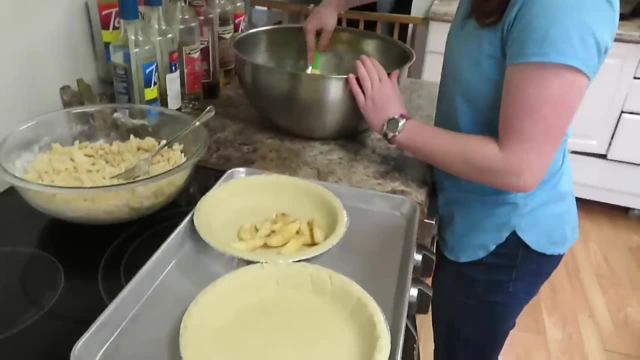 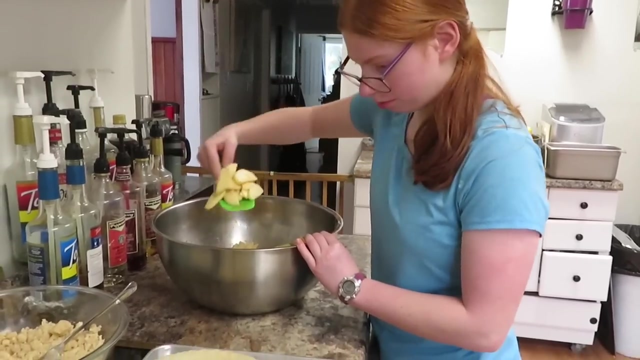 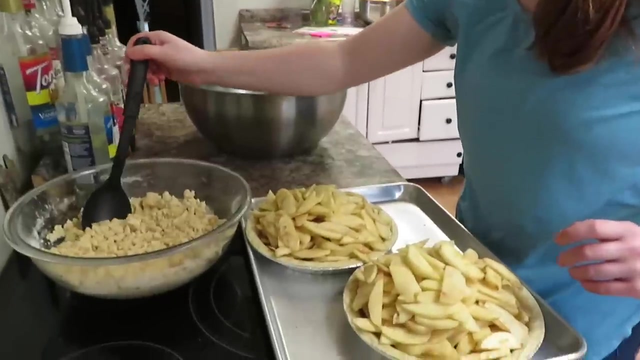 number 11: add apple mixture to pie pan in an even layer. sprinkle come from. make sure on top to cover. so it's gonna be heaped up because as it cooks it's going to cook down. yeah, so it's okay that it's gonna be piled up. so you've divided all your apples up. yeah, now you have to put that. 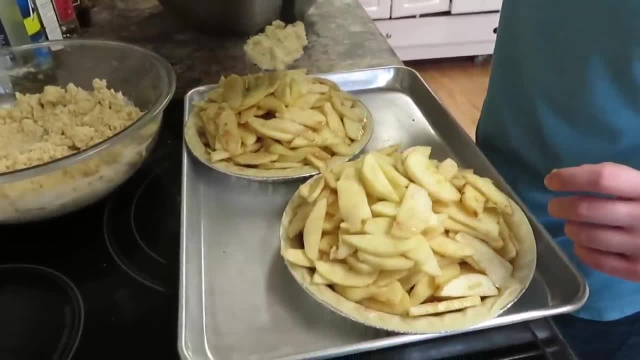 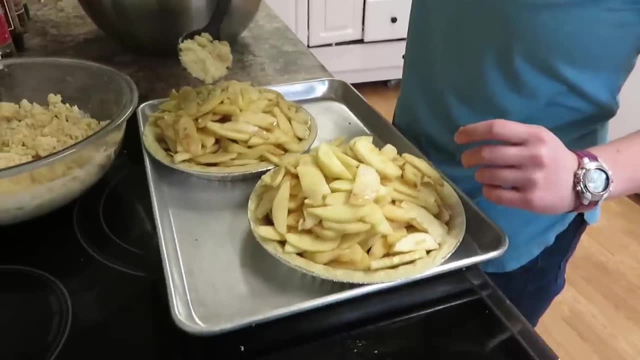 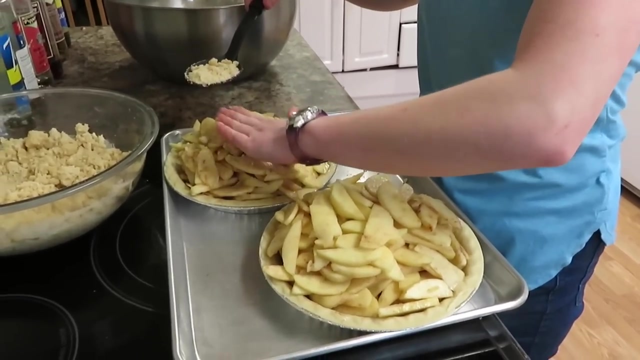 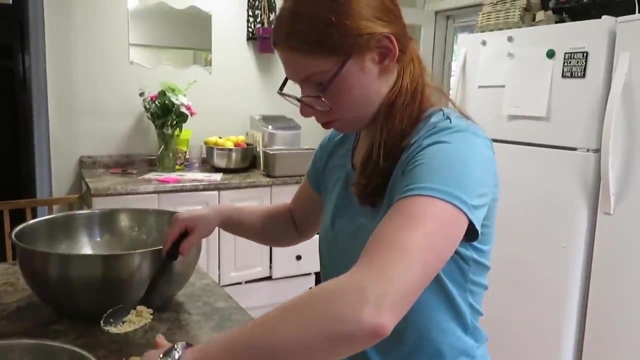 topping on top. so you're trying to make sure that it's going to be evenly distributed. so you're trying to keep it on the pie because otherwise you have more dishes to do, so you might need to use your hand and kind of press it on. it's gonna be a bit more of a challenge because it's a heaped. 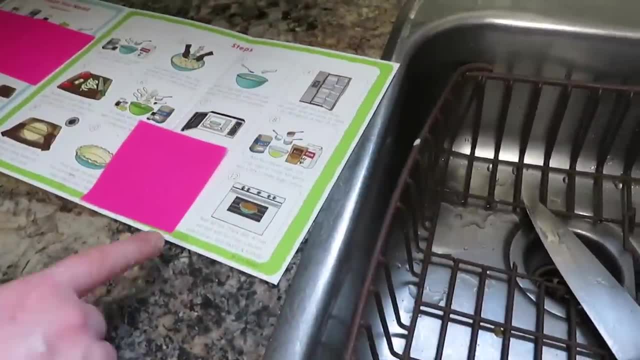 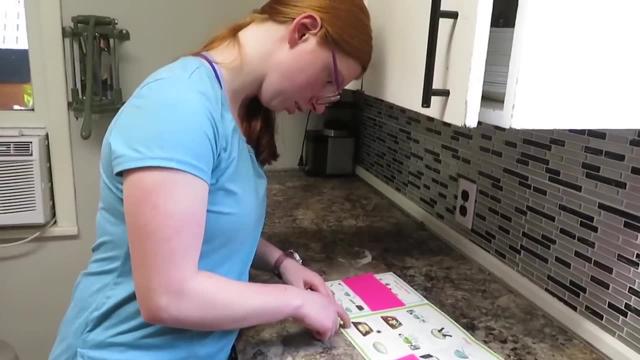 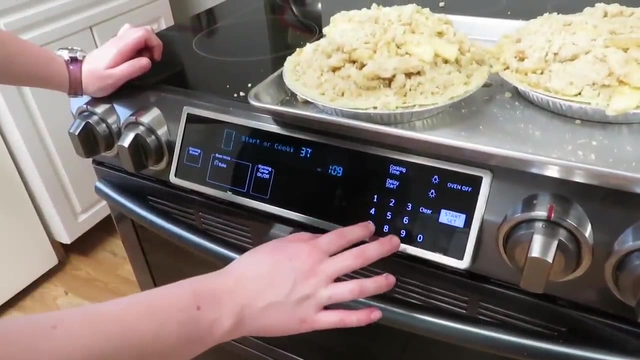 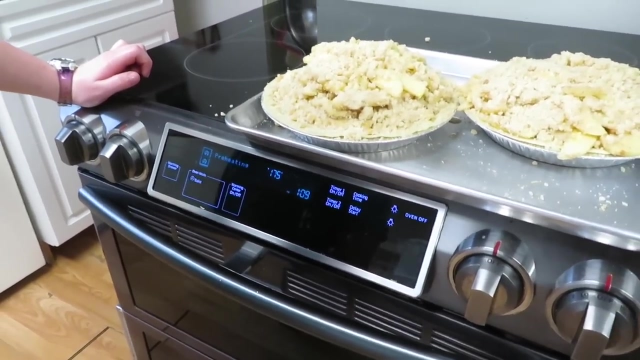 up pie, yeah. so what's next? bake 60 minutes, check after 40 minutes and tent with: well, if top is brown, what temperature? you're gonna cook it up? 375. so bake three, seven, five and start hey, when it comes up to temperature, you're going to put your pies in. okay, so do you think you need? 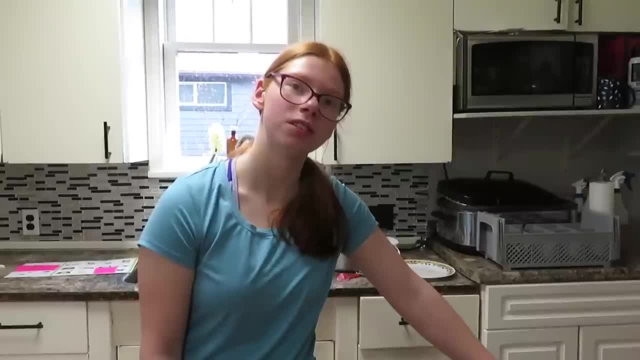 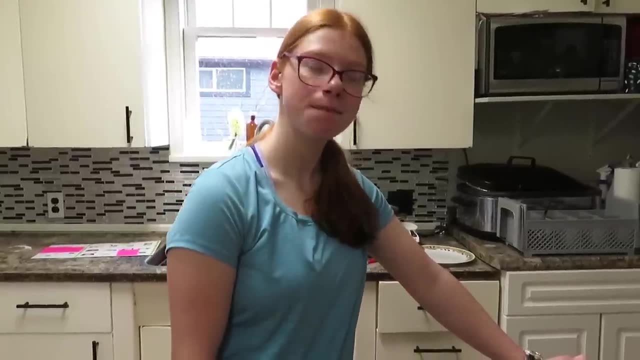 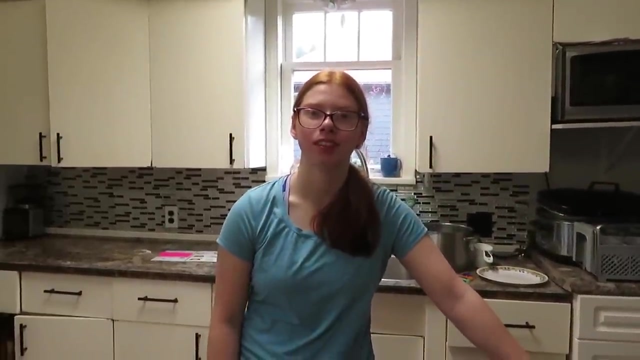 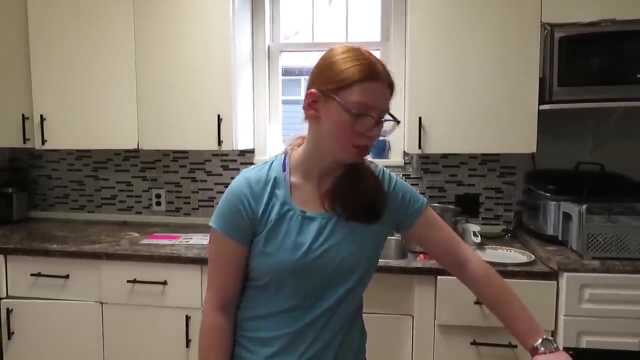 to keep the pan very level, yes, otherwise what's gonna happen? it's gonna end up all over the floor. okay, so we can do some cleanup real quick while it heats up. so your time: you are way past what we thought. oh, okay, so you need to do some speed cleaning while we wait for that to go in the 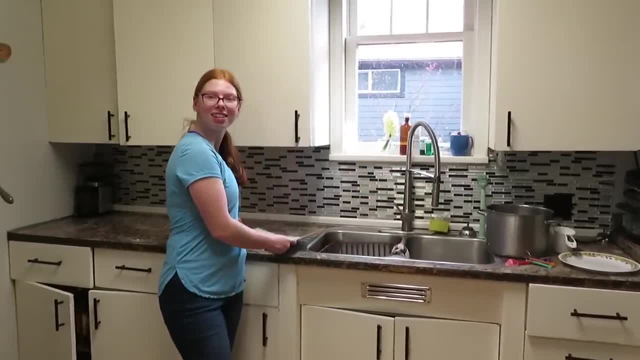 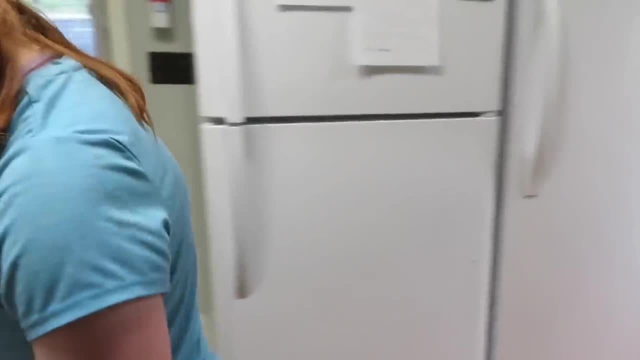 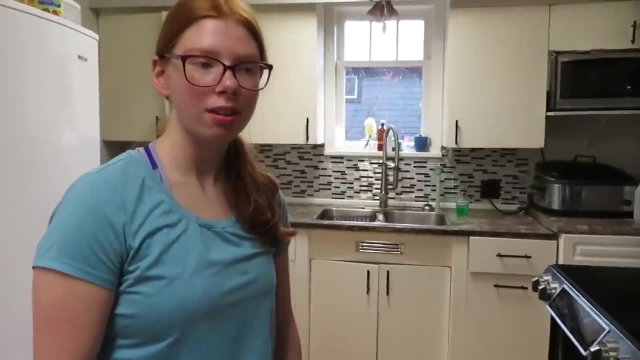 oven, and then we're going to reassess and figure out what we're going to do next. so how long is it going in? for 30 to 60 minutes, I think that's what it said, exactly 40, okay. so what would you be setting your timer at? we're setting the 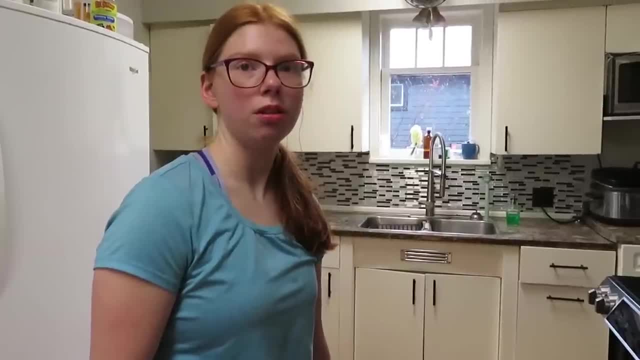 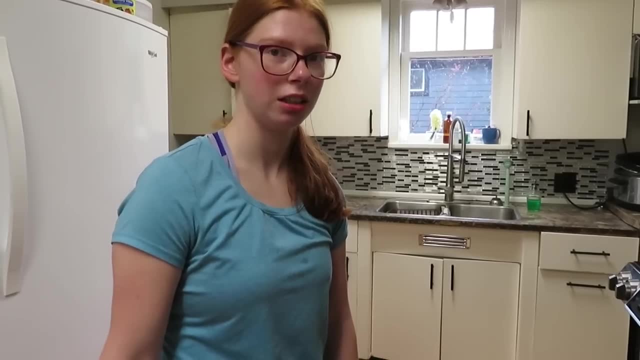 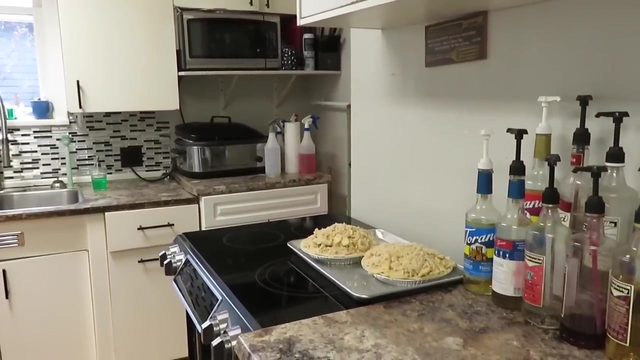 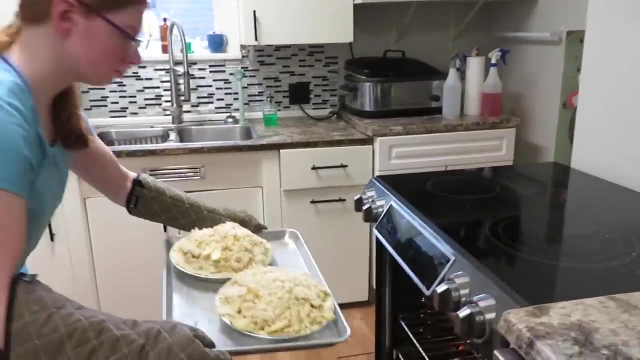 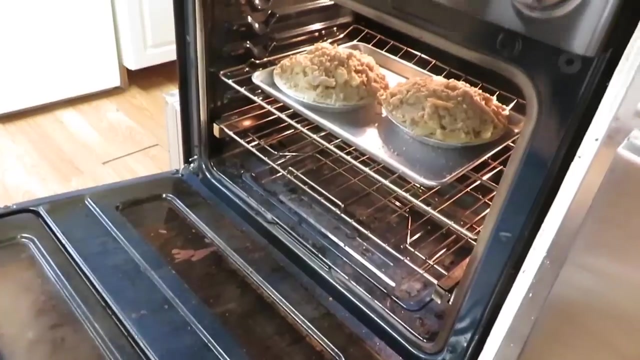 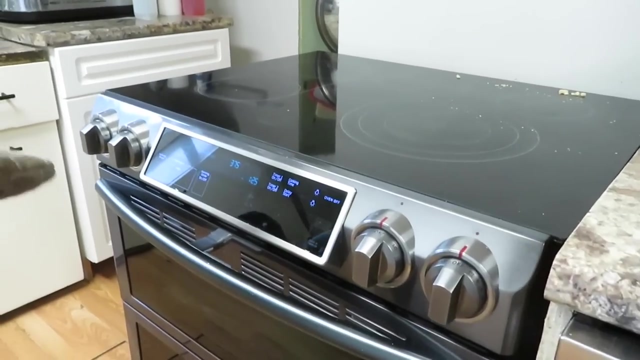 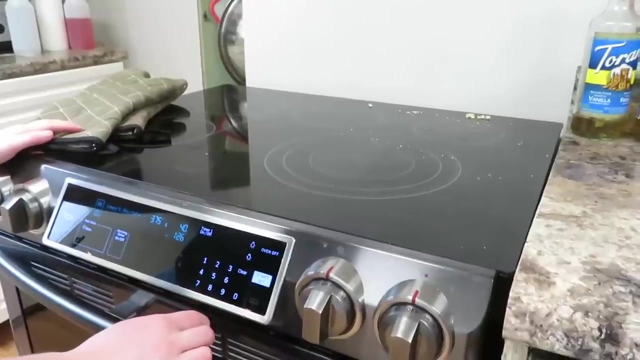 timer. for how many minutes? 60 minutes, but it says to check it at 40. okay, so 40 minutes and then 10 minutes, maybe 20 minutes after that, okay, okay, you set your timer please. so then it's ready for us to go to the next step. 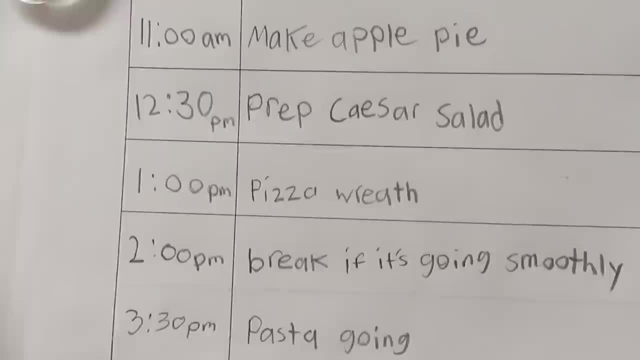 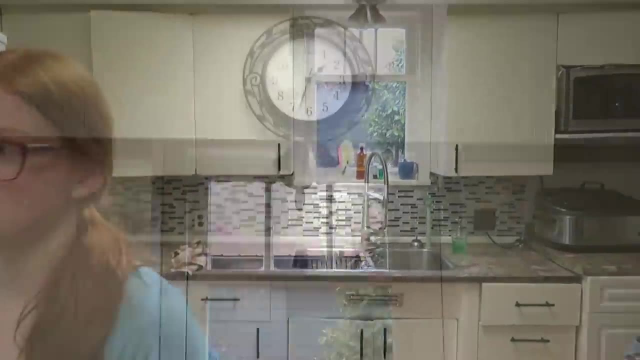 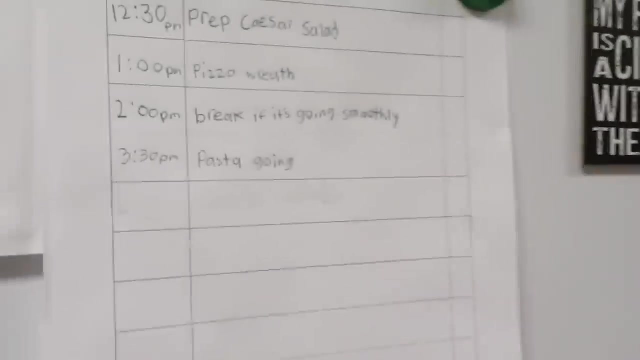 to check at 40 minutes. it will remind us you thought you were going to be done this pie at 1230, yeah, and it is now on 30. so what do you think we should do? do we just keep following our schedule as is, or should we adjust it? I think we. 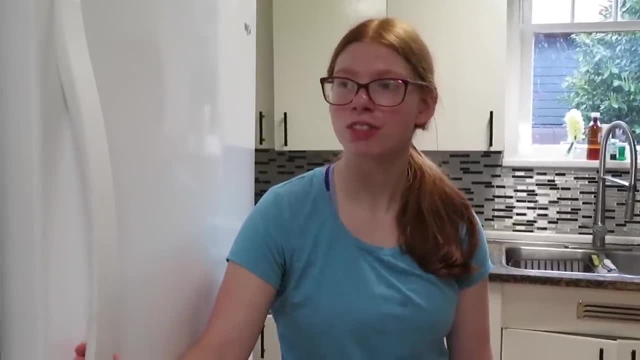 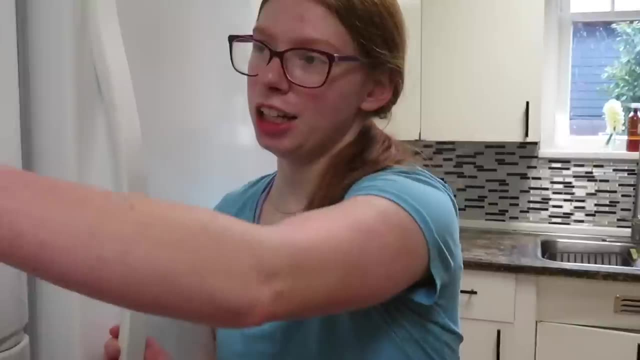 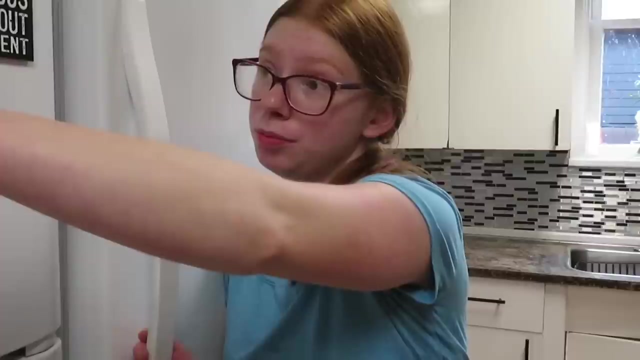 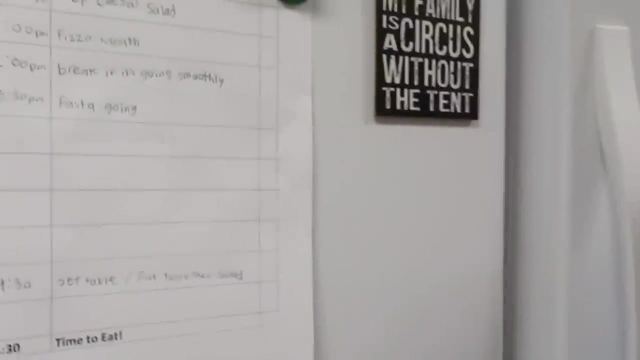 should adjust it. okay, what should we? how should we adjust it? I think, um, it says we should put a break at two o'clock. we should put it at 2: 30 and probably have pizzeria go from 1: 30 to 2: 30. okay, well, we were only going to take a break if 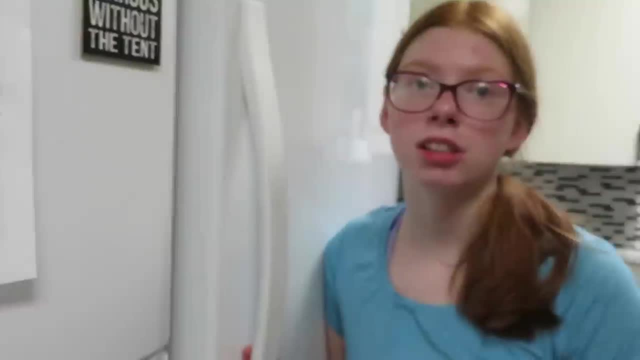 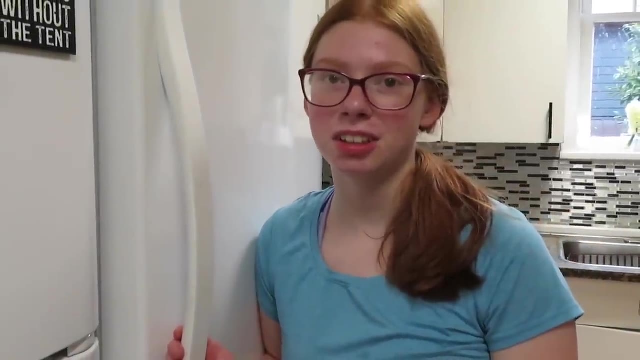 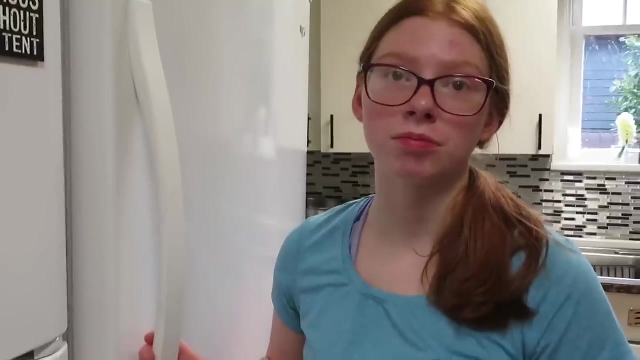 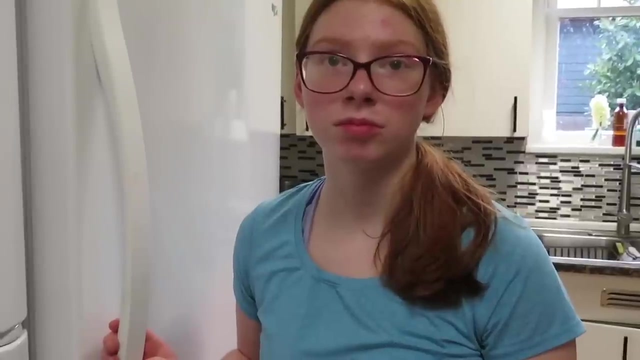 everything was going smoothly- yeah, okay, and it's not going smoothly right now? no, it's going smooth, but we're just running behind. yes, okay. my suggestion is: is we start on the pizzeria, because that's going to take a lot longer than the salad? yeah, okay, and then if that takes too long and we're not ready, 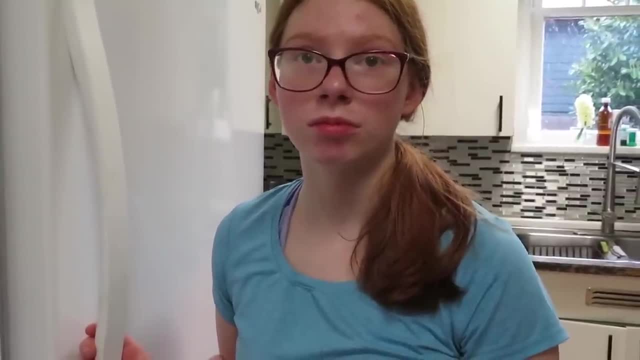 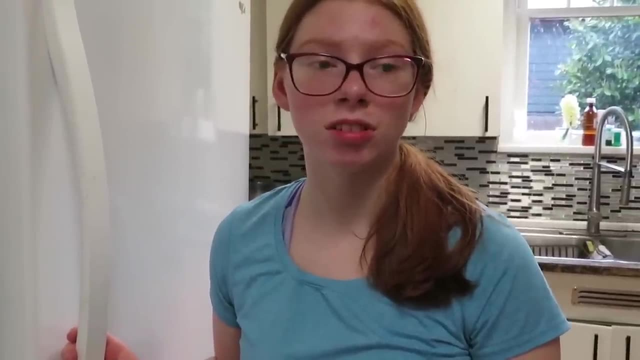 for the at the time. the past is going to be ready. I can make the salad. will you do the pasta? okay, so let's start on the pizzeria. are you going through things in order now? I'm just picking and going. okay, so we have our oven, which is full. 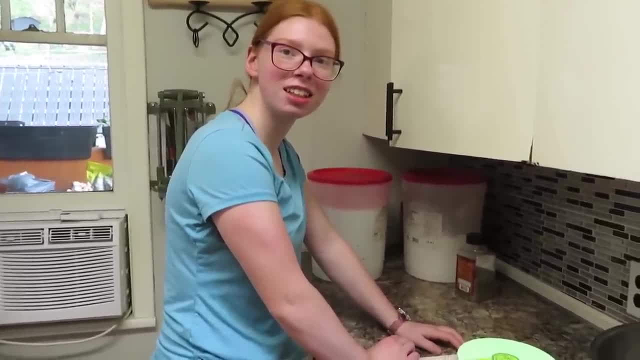 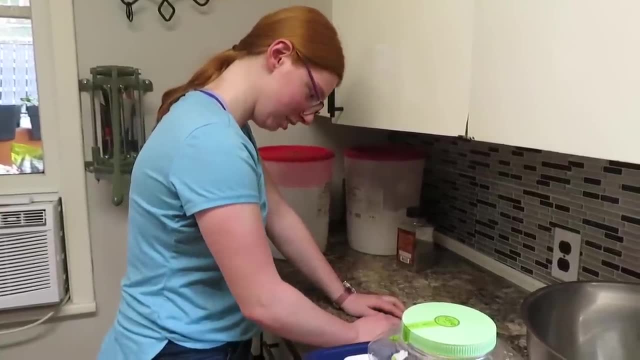 plate. all right, okay, so this is the oven we're using when we totally have all the So is that going to work? because you've been having trouble tracking and keeping track of everything, So would it be best to start at the beginning and work your way through the list? 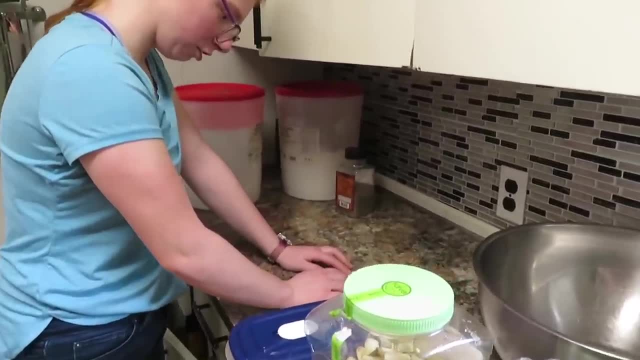 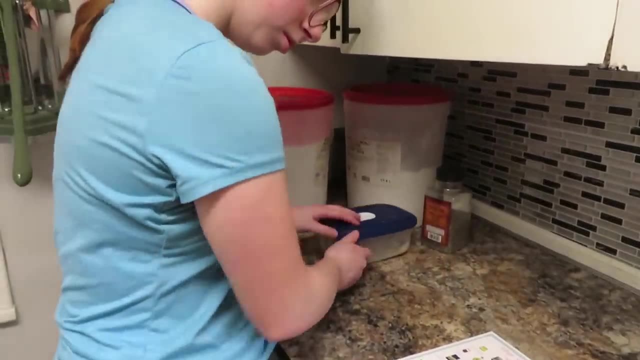 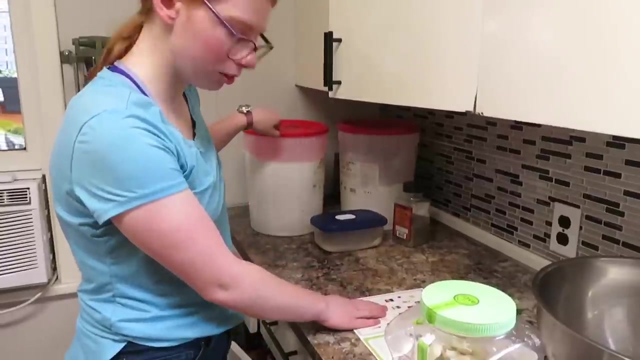 Yes, So what's the first thing? you need Active dry yeast. Okay, so I put the yeast here for you, Okay, Okay, what's the next thing? you need Sugar, which is this one: Okay, Warm water, It's in the tap, so 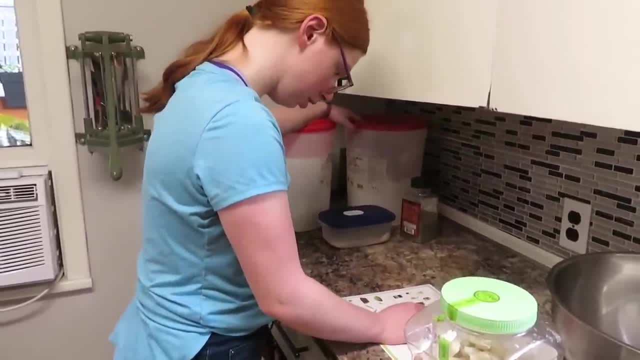 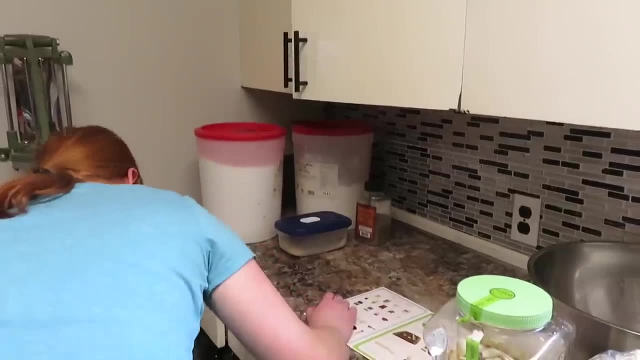 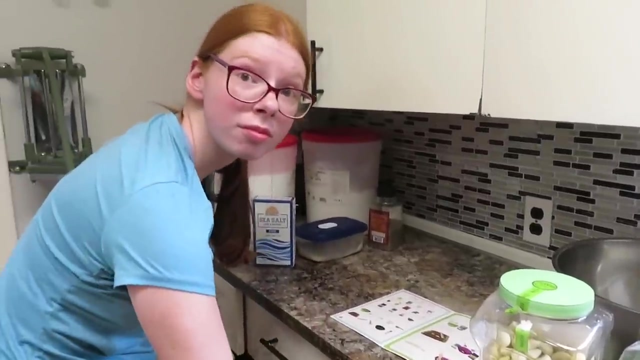 Yeah, And flour is here One salt. Would that be like kosher salt or like table salt, Table salt? Okay, So a little hint. Usually, when they write out the ingredients, that's the order you're going to use them as you're cooking. 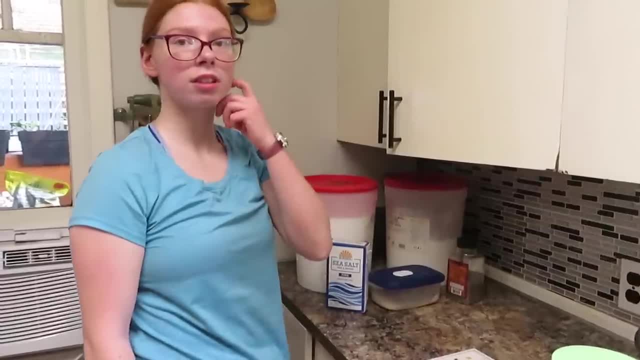 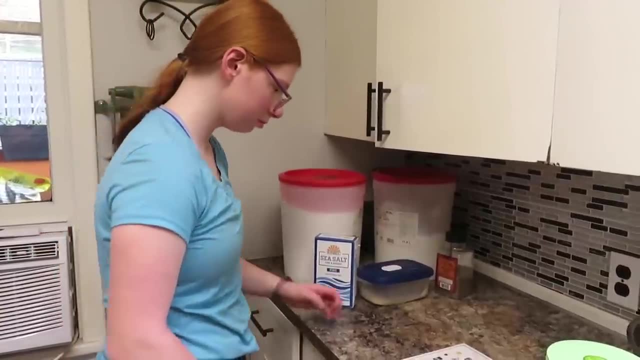 Oh, okay, Okay, so if you start at the beginning and work your way through as you're collecting them, okay, And keep them in some sort of order, they're going to be the same order you're going to knead them. 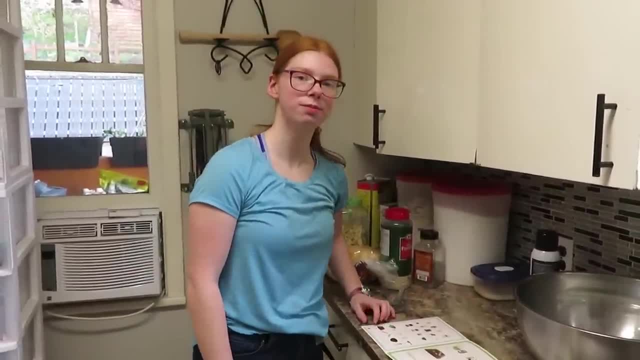 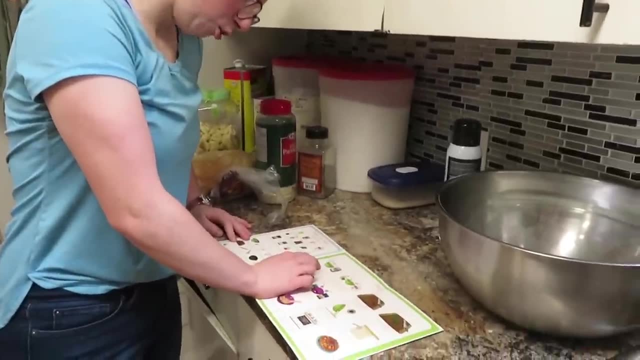 Okay, I have all the ingredients and I have all the utensil stuff, So are you ready to start? Yep, Okay, what does step number one say? Make no-knead pizza dough, Mix yeast, sugar and warm water in large bowl. 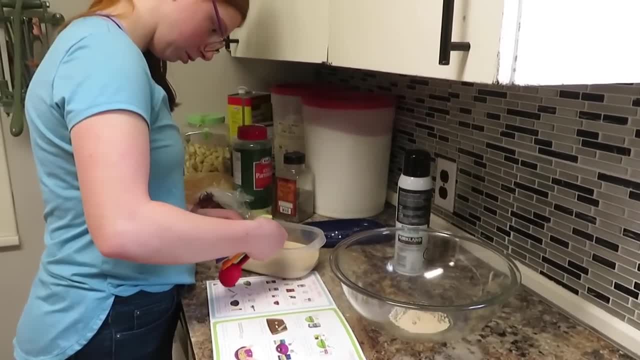 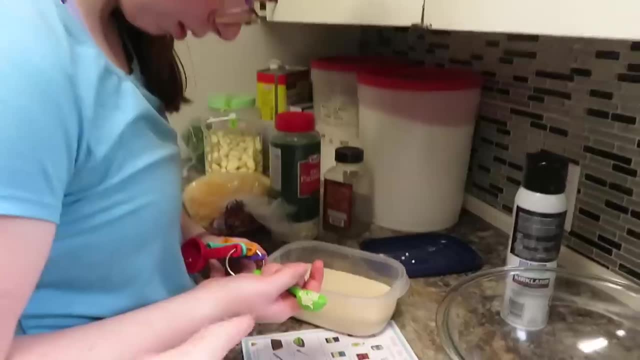 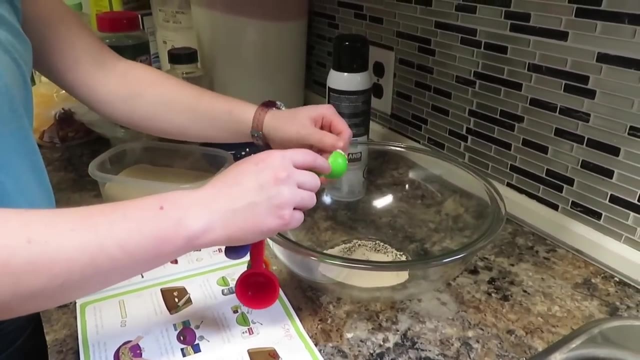 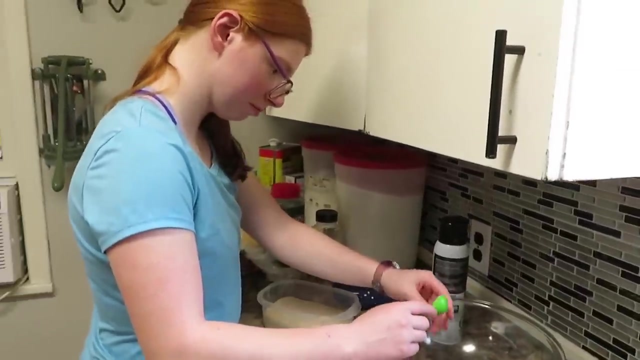 Make sure it's filled up right up. Okay, you have a lot stuck to here, So that's actually the ingredients that you measured. So it's important that your spoons are dry when you're scooping up dry things, Because otherwise your measurement isn't correct anymore. 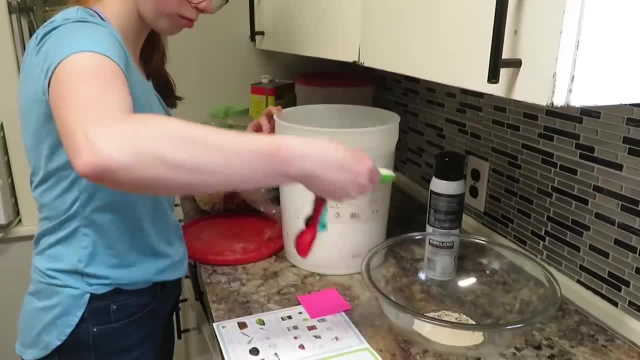 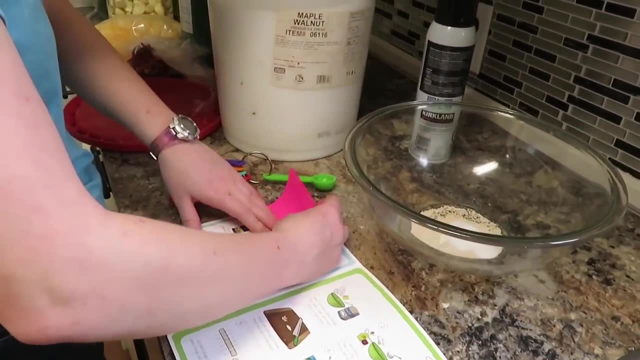 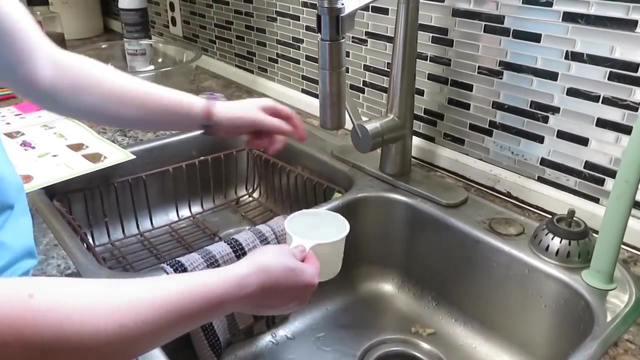 Wesley's, Move your paper over to make it easier for you. One cup more Right up, Okay, so right now you're going to go ahead and get ready to start the dough. So you're going to do that with the flour and you're going to add the eggs and drink it up all at once. 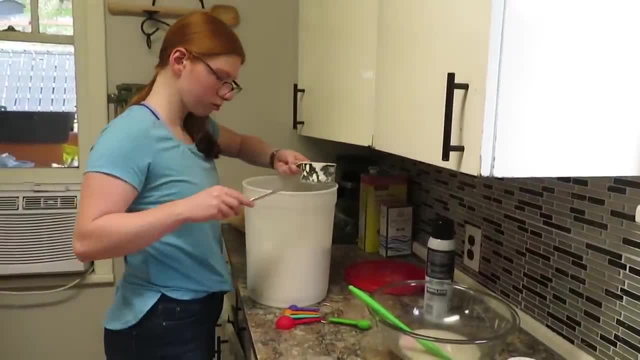 Okay, Okay, so I'm going to add the rest of the water and then I'm going to add the yeast in here. All right, All right. Okay, so I'm going to pour it in. All right, All right. 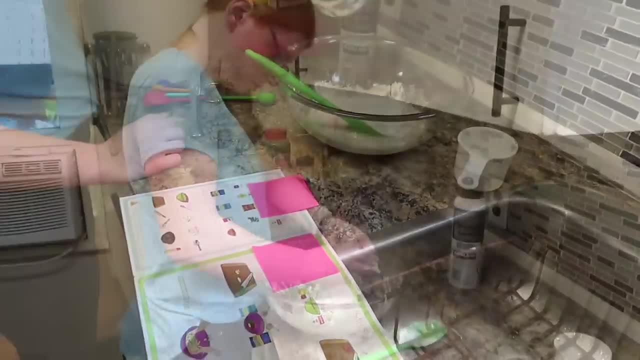 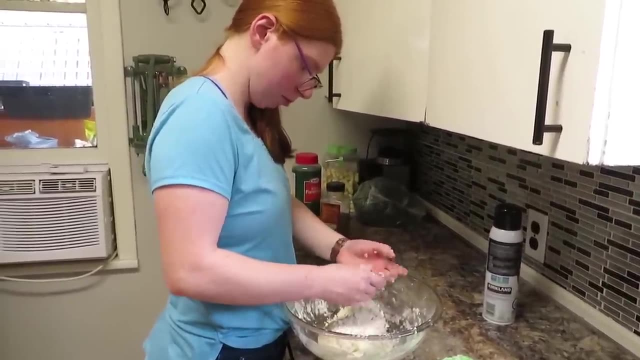 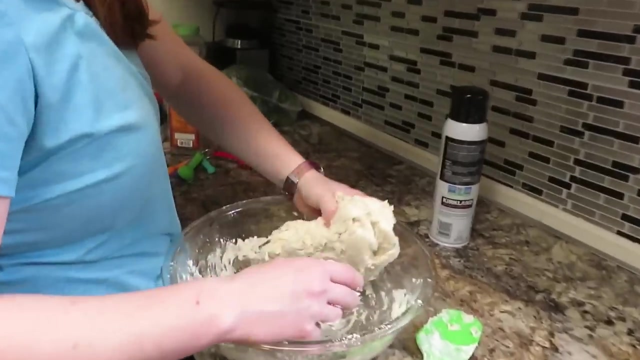 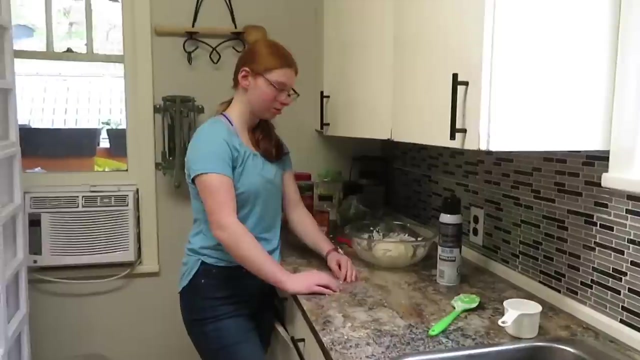 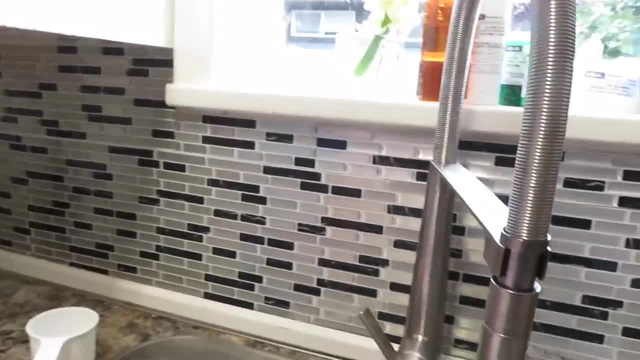 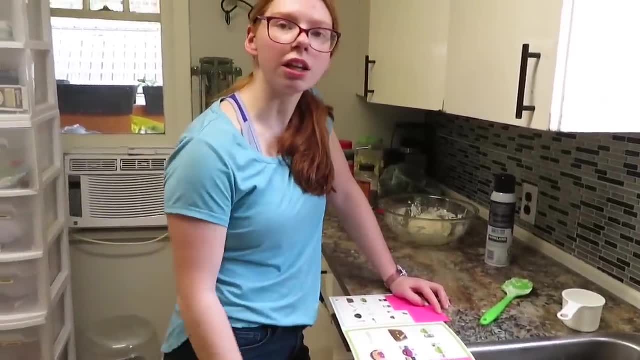 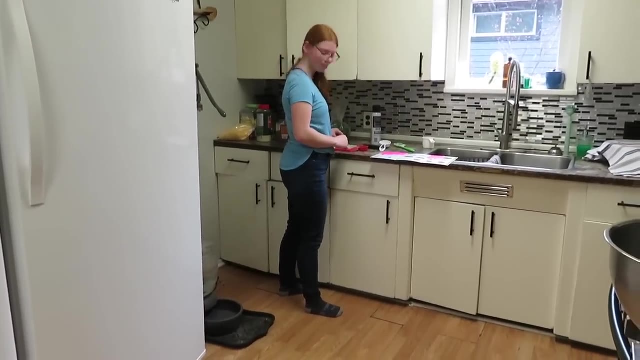 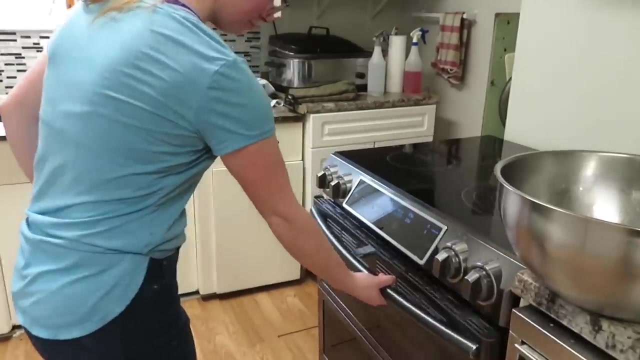 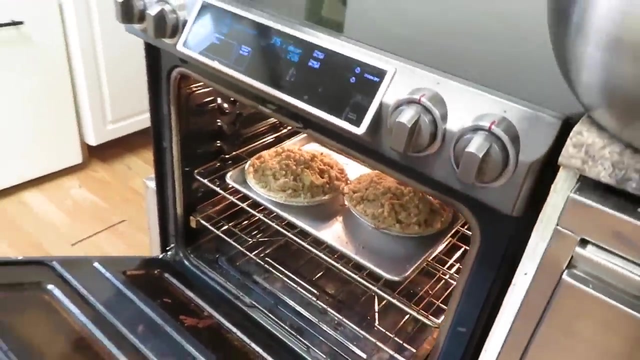 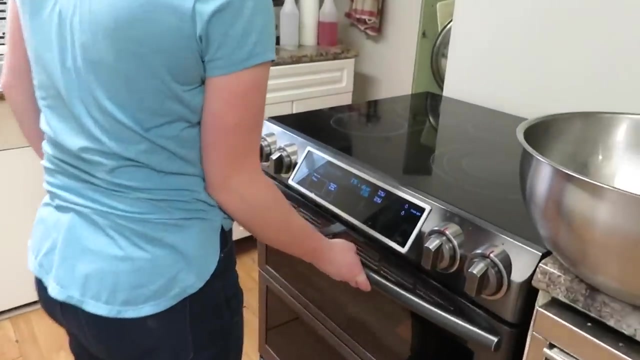 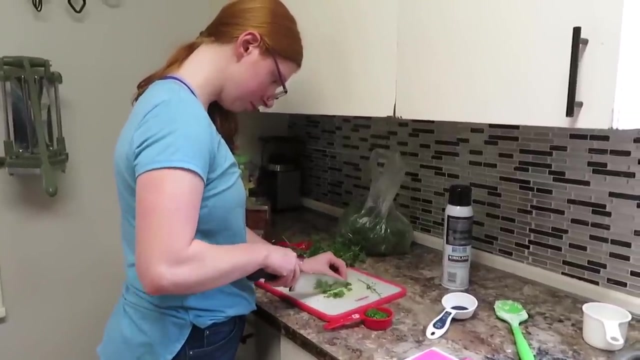 that 10 minutes so they could finally mince parsley to make one fourth cup and then add with cheese. okay, so you can start chopping up your parsley Cheyenne. I hear a timer going off. what is that? okay, I'd say it needs the next 20 minutes, okay. yes, when you're cooking multiple things, even if. 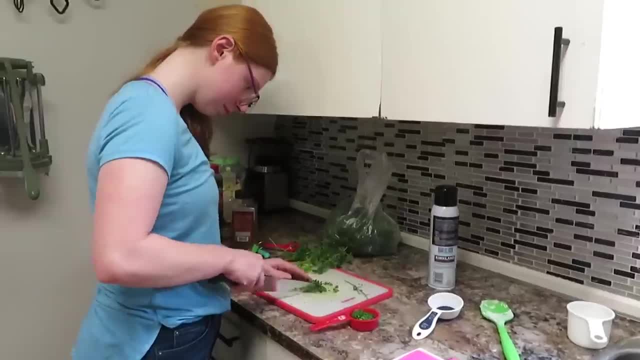 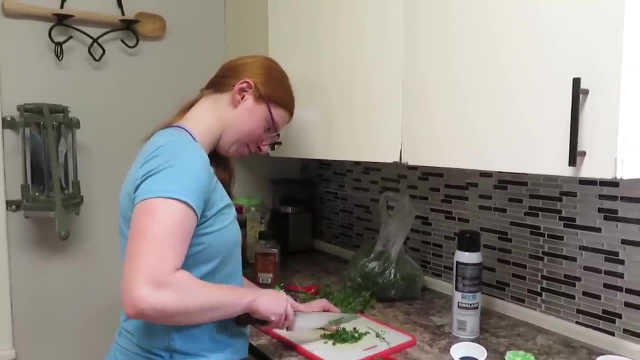 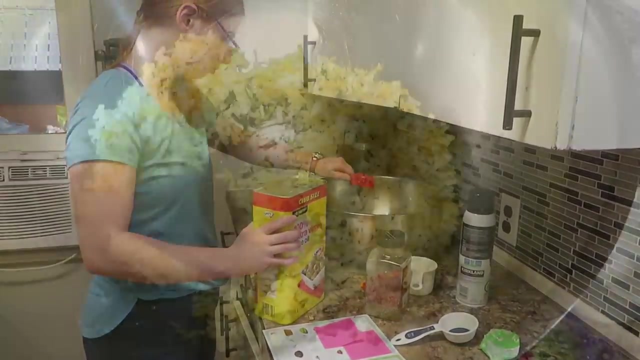 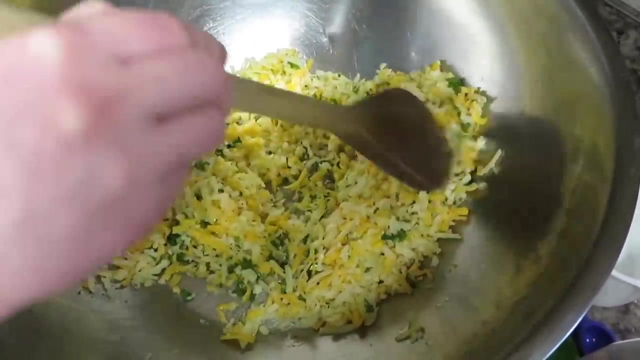 you're busy doing something, your timer starts going off. you can't just pretend you didn't hear it, okay? hmm, because your pie could be burning and then you would be further behind. that is gonna make the bread taste so good. yep, it got big. did it grow before? I was like half the 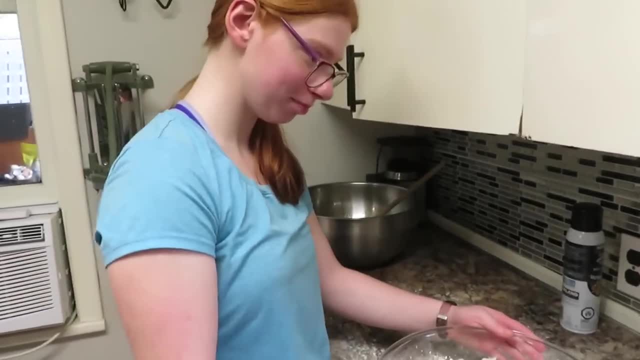 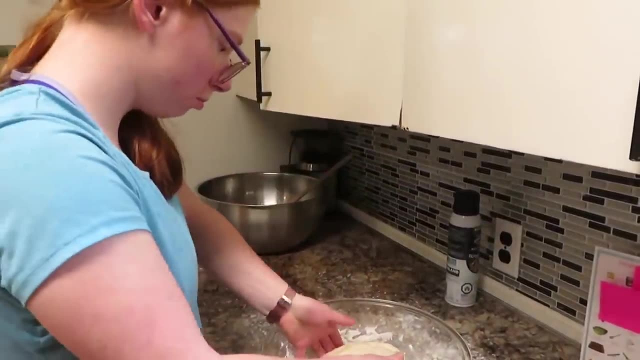 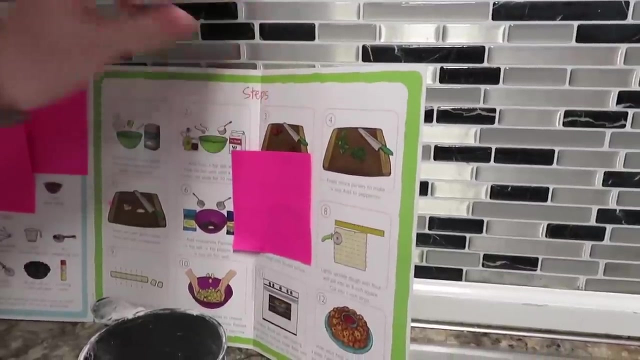 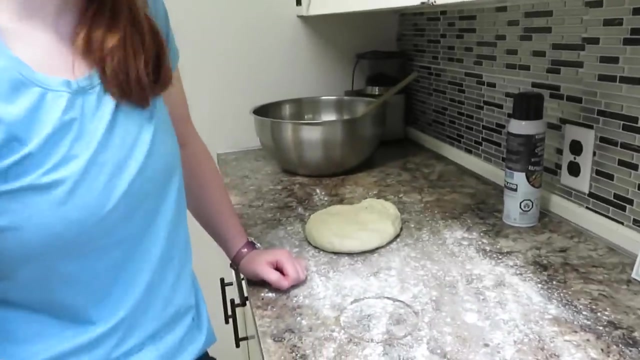 size. yeah, and it doubled. yeah, okay, what do we have to do with it? we have to pour dough onto a flat surface, okay. lightly sprinkle dough with flour and pat into eight inch square. cut into one inch strips, okay, so flatten it out and try and make it into a square. 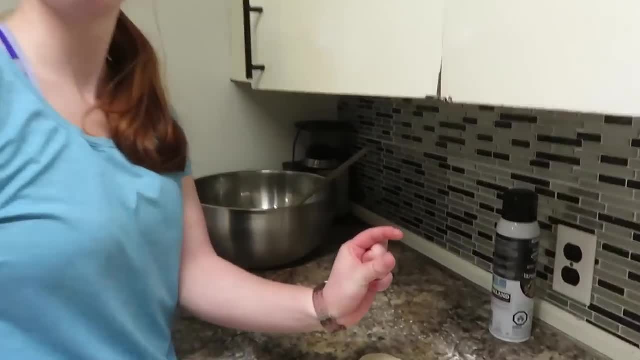 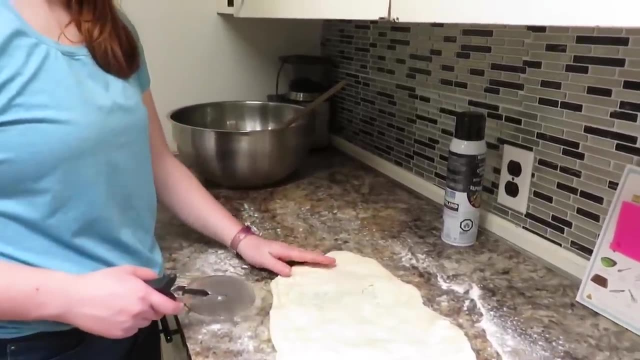 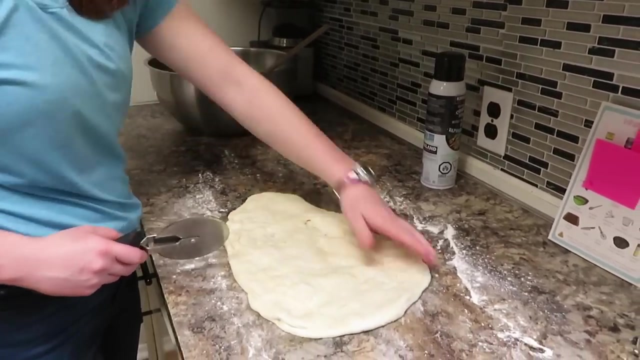 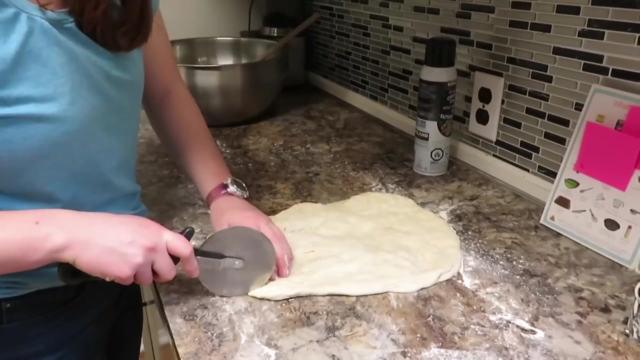 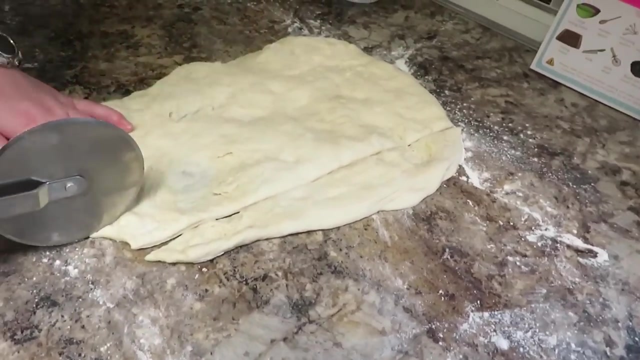 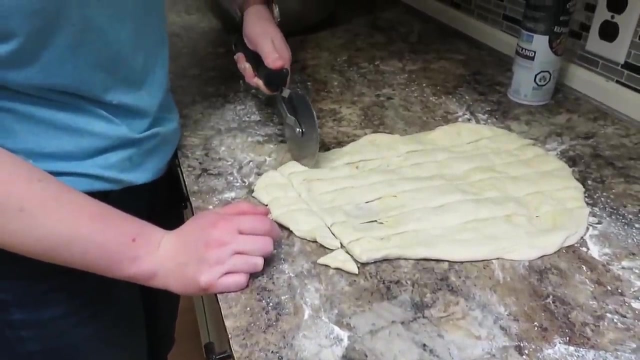 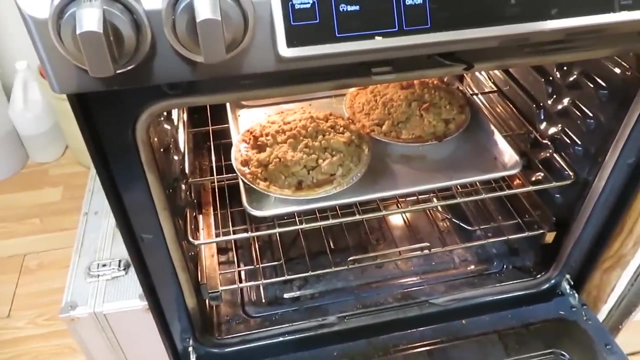 as big as one inch, my method. okay, so you're making it into small little squares, right? so we're going to make a strip and then cut that strip small. okay, should I cut it lengthwise or whatever way you would like, right there? sure, look at your pie, it looks done. 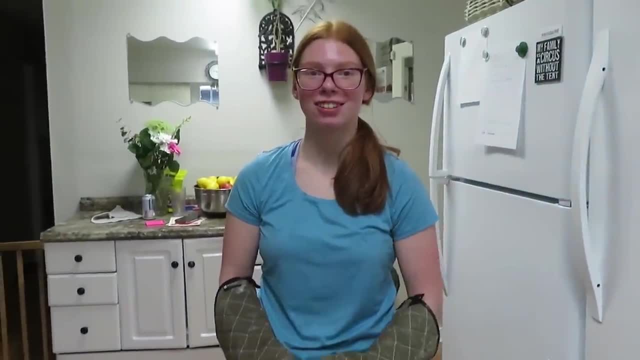 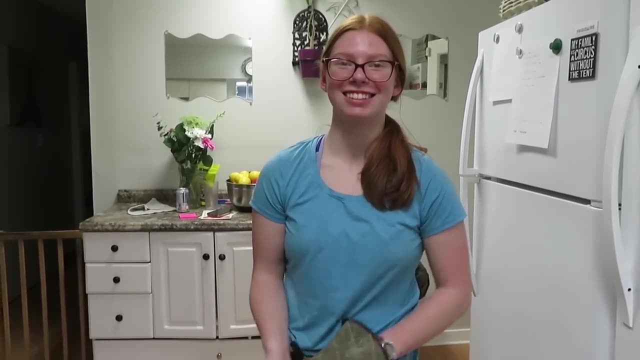 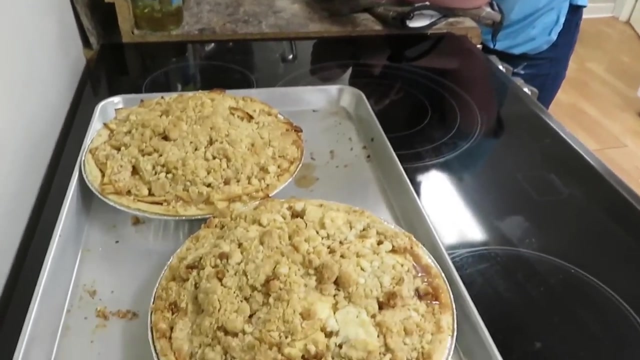 so you're going to need to carefully lift this out. okay, are you feeling confident enough to do this, or do you want me to? I want you to do this. I might end it up all over the floor. that wouldn't be any good. okay, I will do it. that looks delicious. it does look very good. 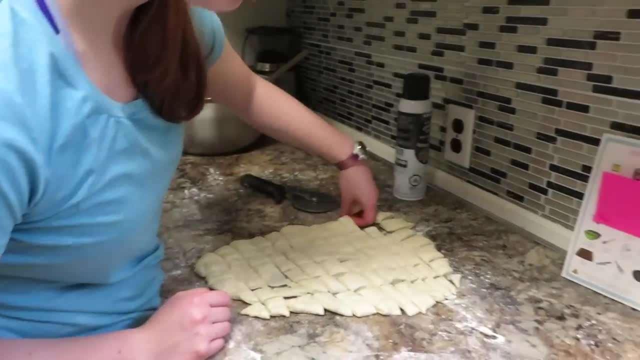 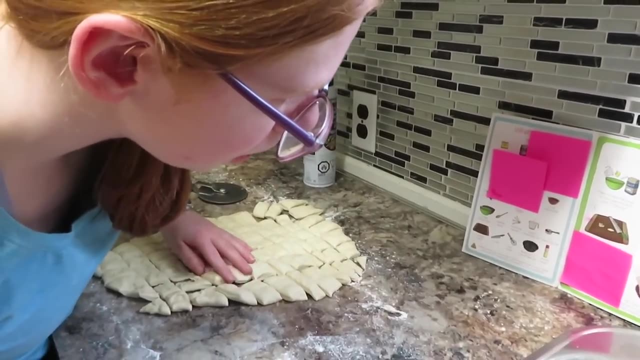 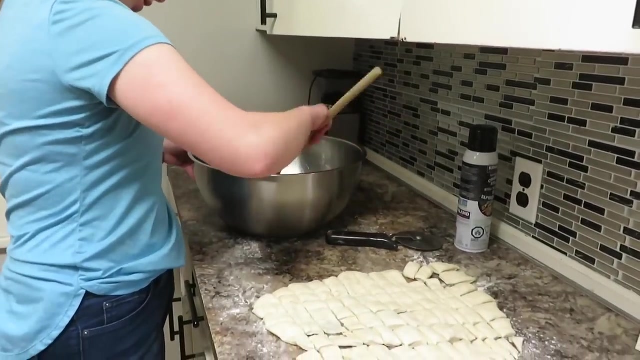 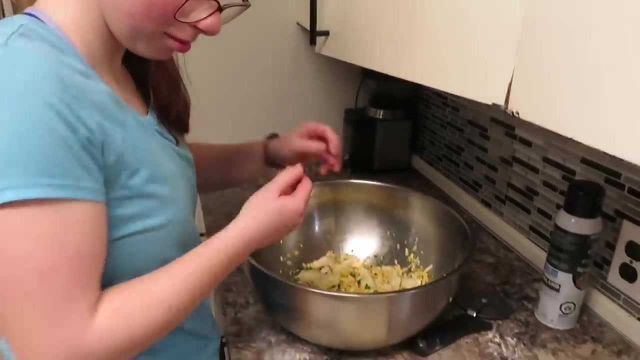 so they're all cut. yep, what does it say to do? add a few dough pieces of cheese mixture, toss gently with hands- repeat with meaning, though do not over mix. okay, so you're gently covering them with your cheese mixture- and add the resting, so they're all mixed in. 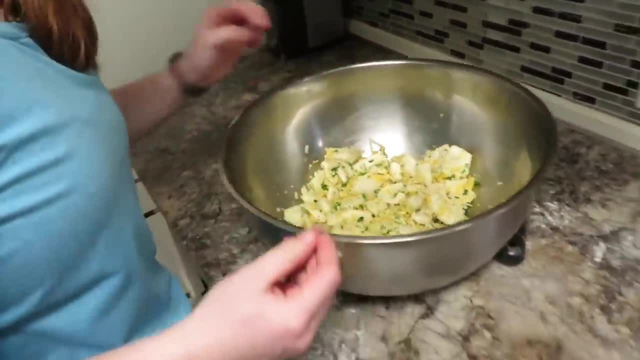 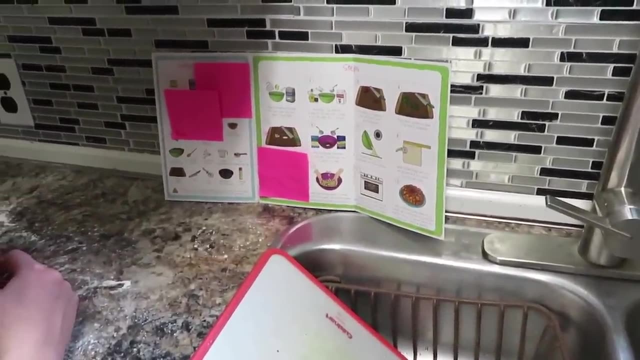 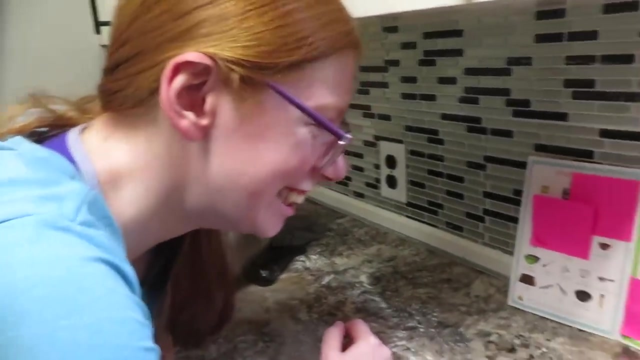 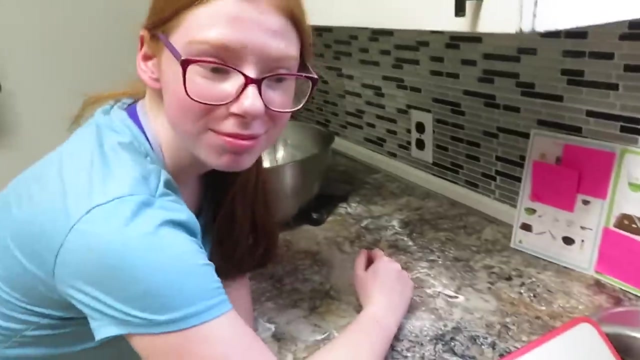 what's the next step? let's take a look. grease bandit pan with cooking spray. grease Bunt pan. scoop mixture- I like your way better. bandit pan, thanks. scoop mixture inside. Bake until golden brown about 30 minutes. okay, perfect timing, because your pies just came out of the oven. 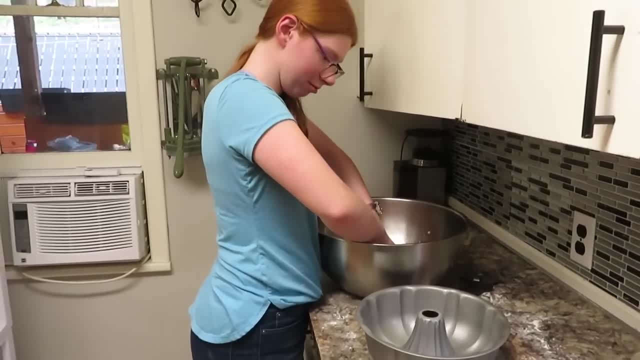 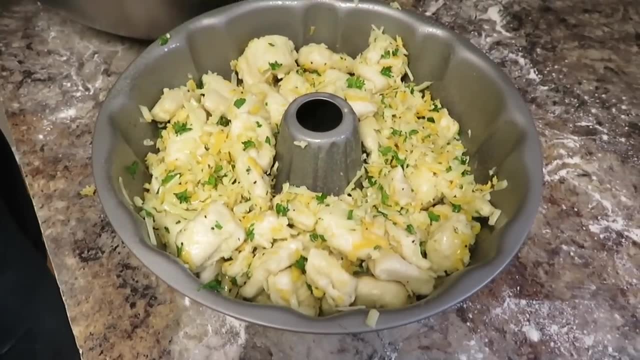 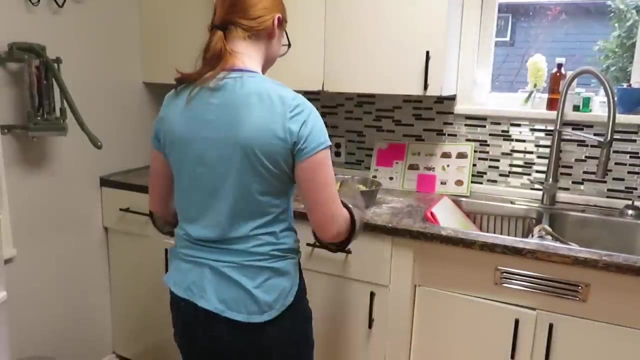 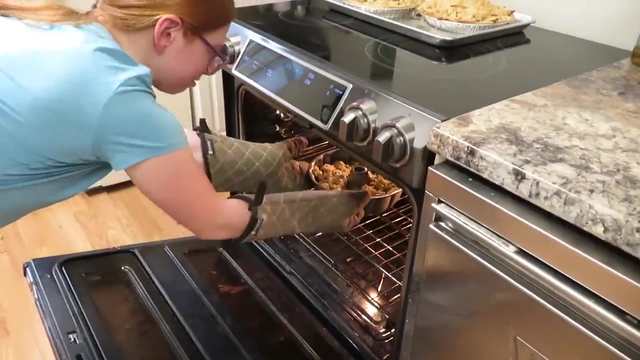 I already greased that for you, So you just have to put it all around the edges. It's looking really good. It smells delicious. Can't go wrong with Garlic and cheese Recipe number two towards dinner. Yep, Halfway there. Everybody's going to be so Full after supper. 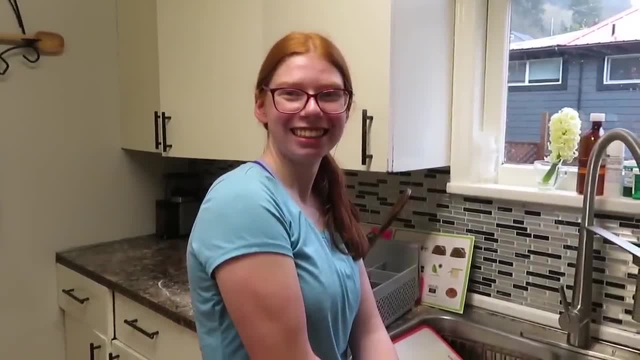 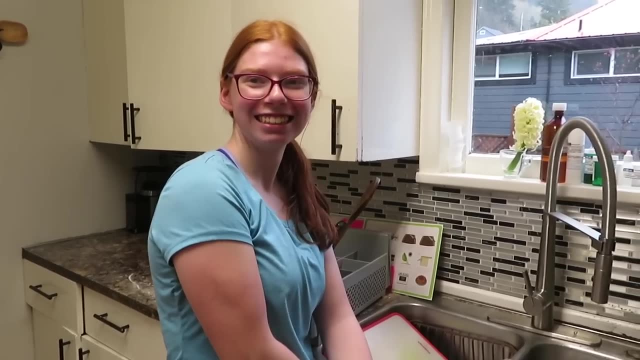 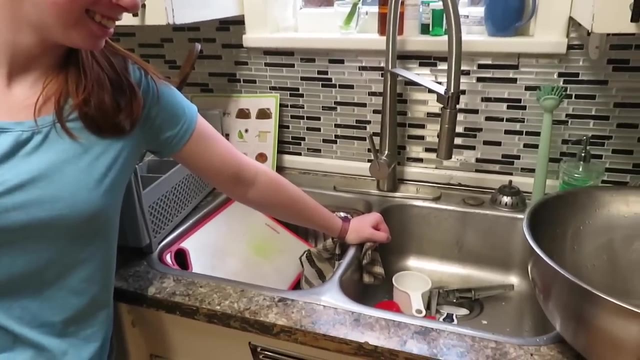 I think so. I think you're kind of torturing them Because it's been smelling so good All day so far. But they're just like: I'm hungry, let's eat now. So we're going to get these dishes done And then we're going to re-evaluate. 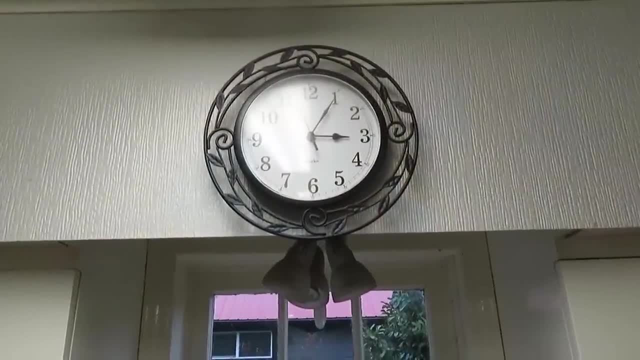 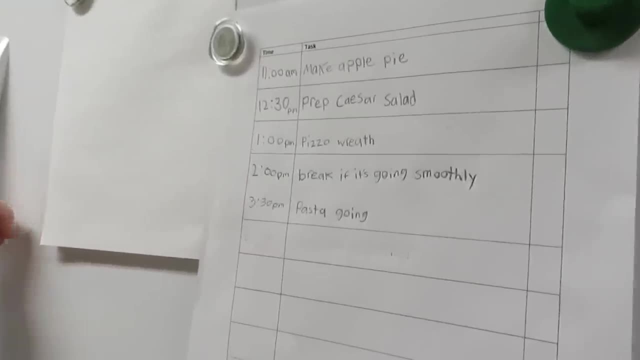 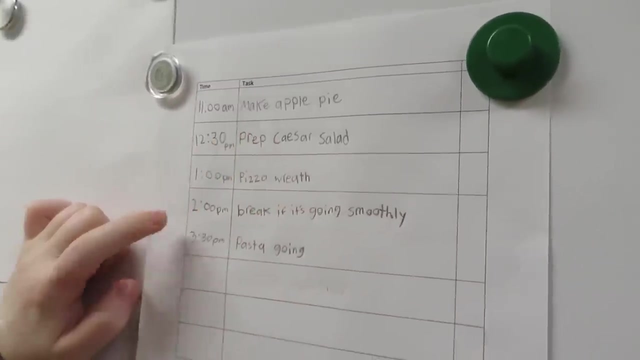 Our schedule and see where we're at. It's three o'clock. Where should we be on the schedule? We should be Still having our break. Okay, So your pizza wreath is cooking. We still haven't done your salad, Or the pasta. Or the pasta. Do you think that we can get the salad done? 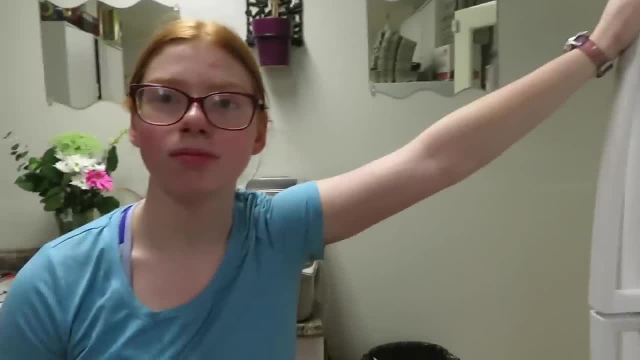 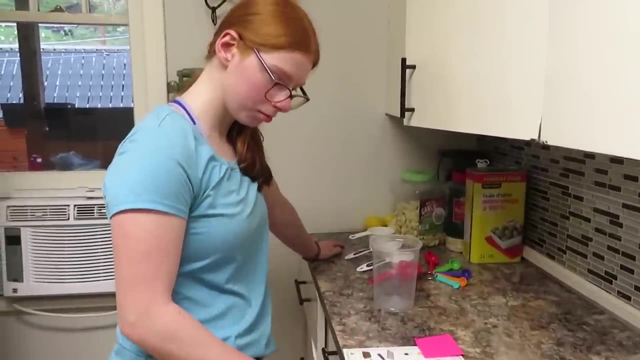 By three thirty, And then we will be back on track For doing the pasta. Okay, let's get it done. So we are going to make up the salad dressing In that pot And put it in the fridge, And then we're going to cut up Your lettuce and kale. 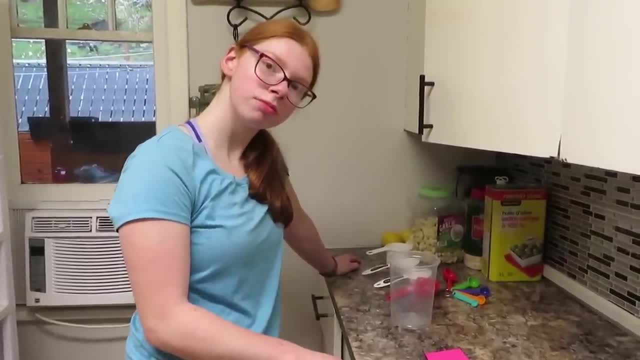 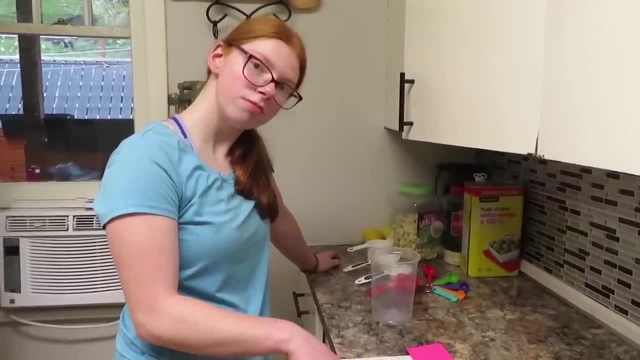 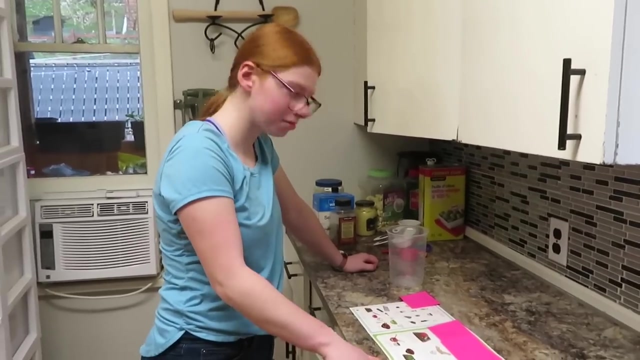 And have it in a bowl And we'll put a towel over it And keep it In the fridge And then That'll be ready, Because all we'll have to do right before dinner Is mix it together. Be all ready to go. Do you have all the ingredients for the dressing? 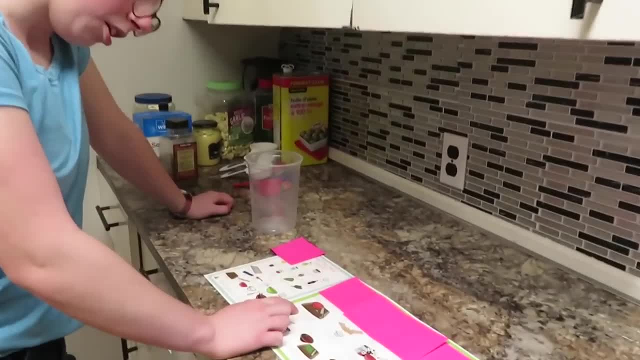 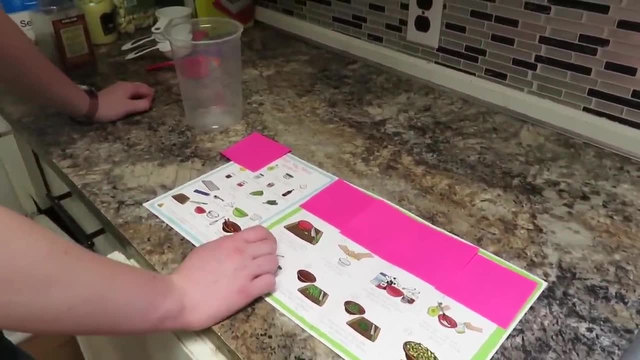 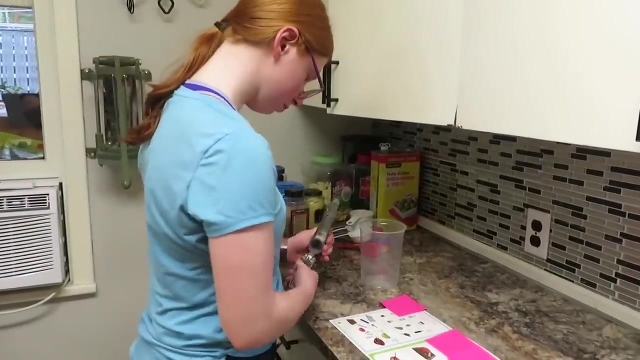 Yes, What does it say to do first, Step five: Meanwhile, prepare dressing, Smash and peel garlic Mince and add. That's a small bowl. So get your garlic press And crush your garlic And we're going to do it in this pot. Okay, So that it can just go directly into the fridge. 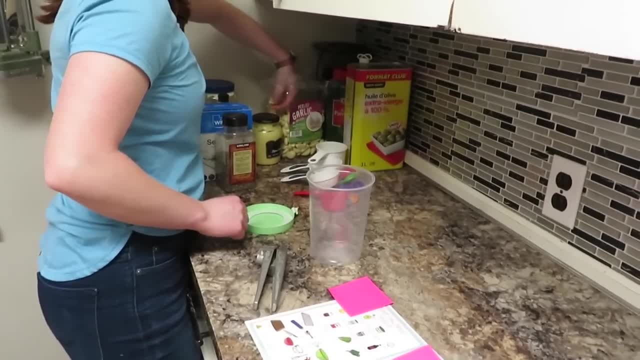 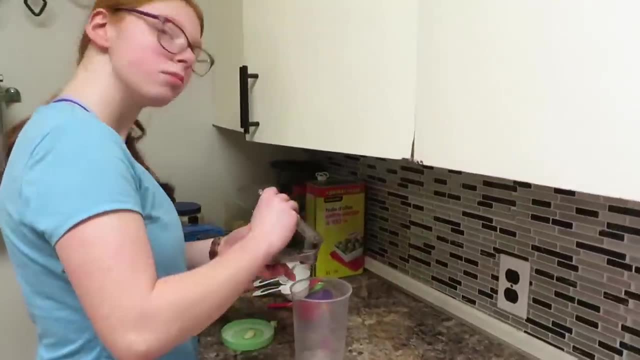 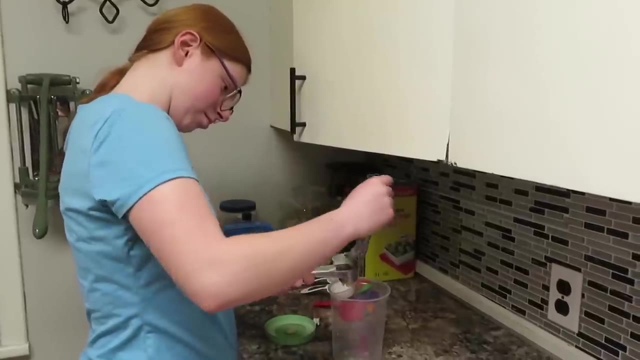 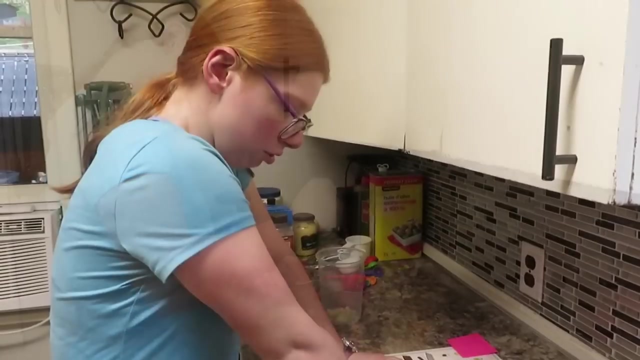 Okay, We only need two. This Caesar salad is one of our favorites, isn't it? Mhmm, I personally could eat it. I could eat this Caesar salad for every meal. When did you get sick of it? I don't think so. It's so good Juice lemons. 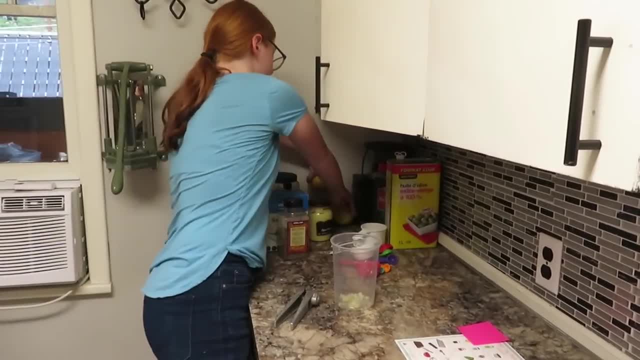 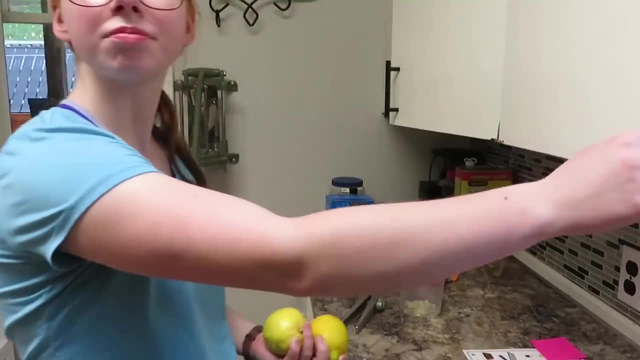 Okay. so you need to cut those lemons in half And then you have to squeeze all the juice out. You might want to do it into a separate bowl, Because sometimes there's seeds, So would a cereal bowl be okay? Yes, We don't want seeds in our dressing. 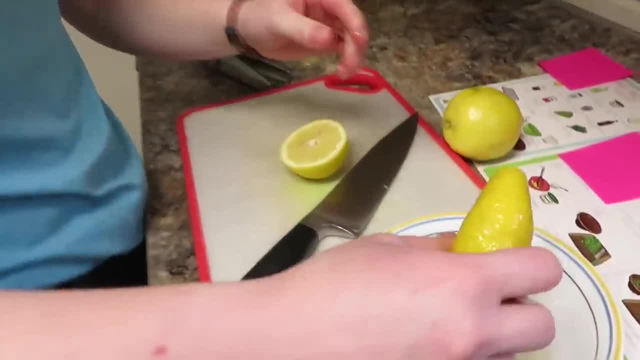 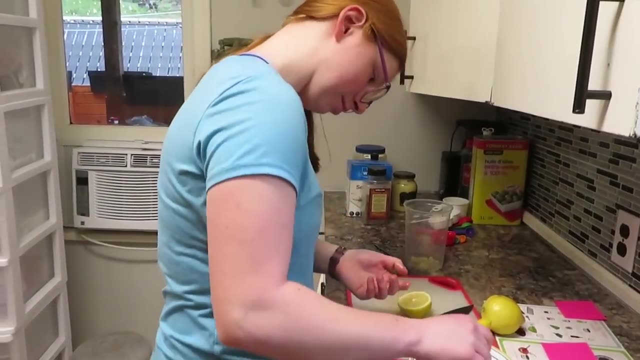 You were right about the seeds. How many seeds do we need to put in our dressing? We don't want any seeds in our dressing. How many seeds do you have? Like ten From half a lemon? Mhmm, and there's still another one. So what's harder to squeeze, garlic or lemons? 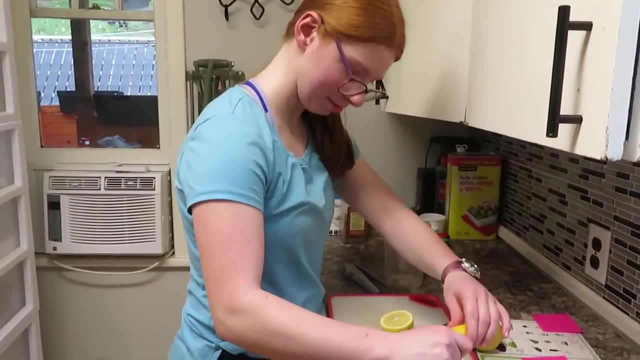 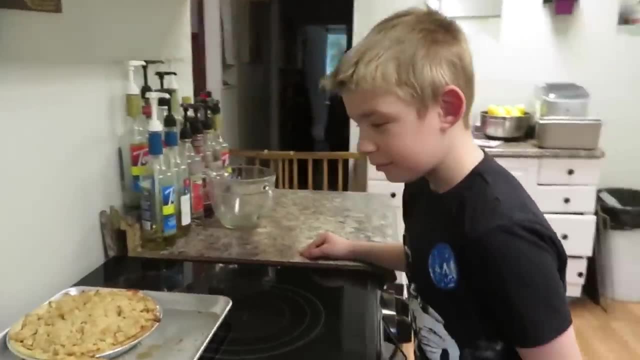 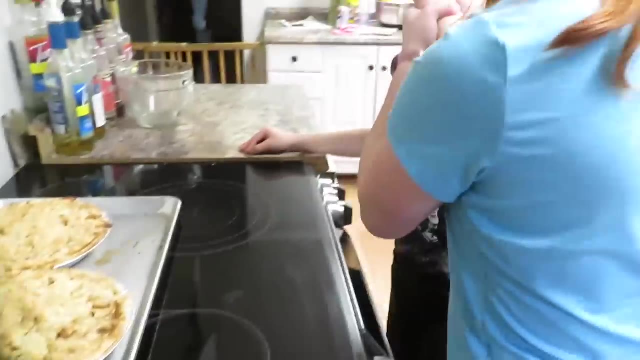 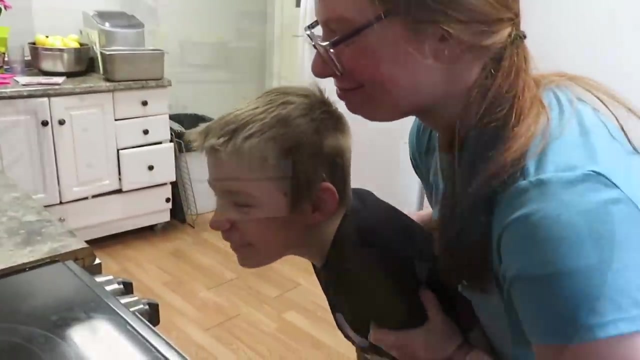 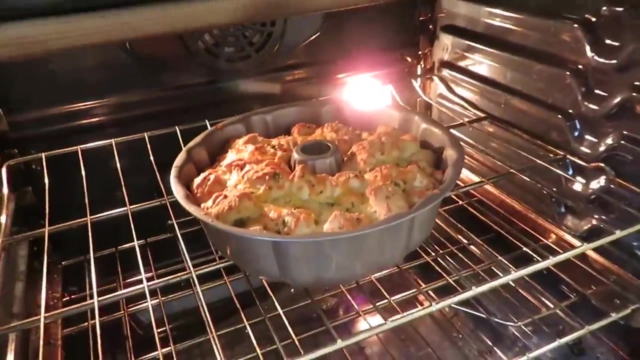 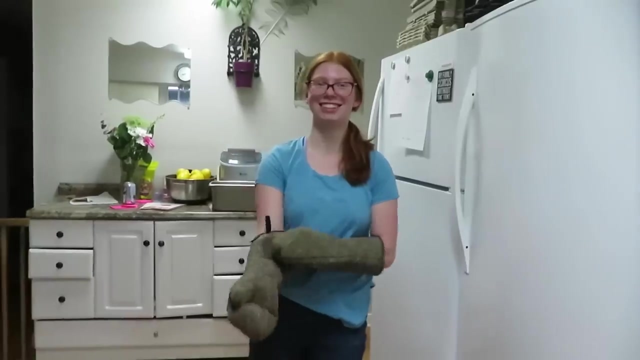 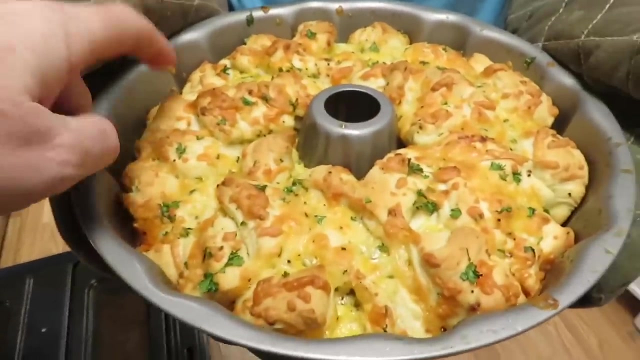 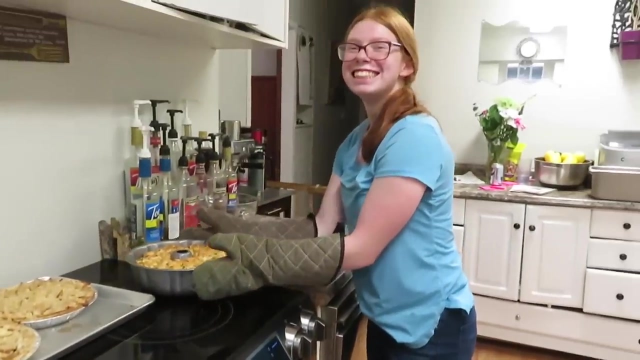 Lemons, because they're really wet Once you squeeze them And you want to get all that juice out. No eating, And I only have one pie for mom, One pie for me and one for you, Lucas. No, No, No, No, because we'd probably eat it all before dinner. 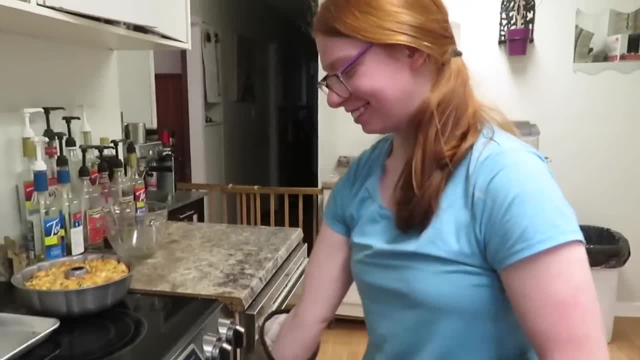 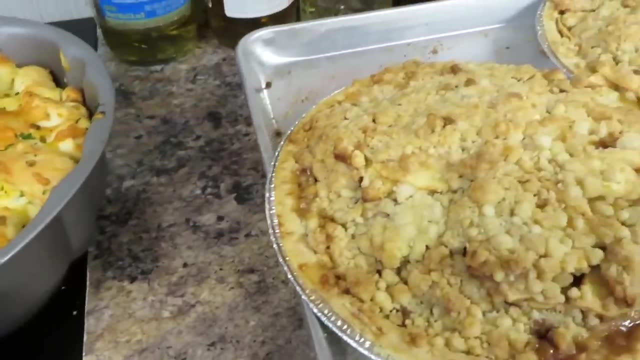 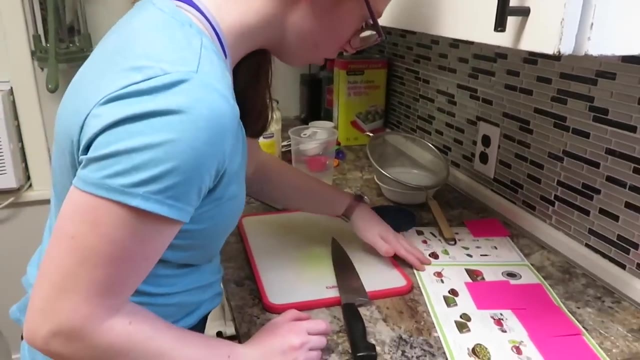 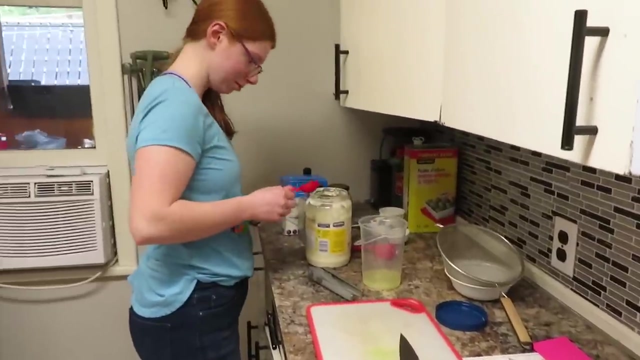 It would be like yours and my snack And nobody else would get any Time for mayonnaise. Let's see how much mayonnaise: Two tablespoons, Times two, Four. Okay, You're going to be a math freak. You're going to be a math pro by the end of today. 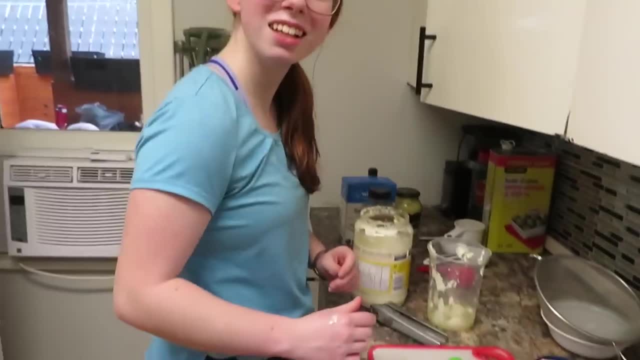 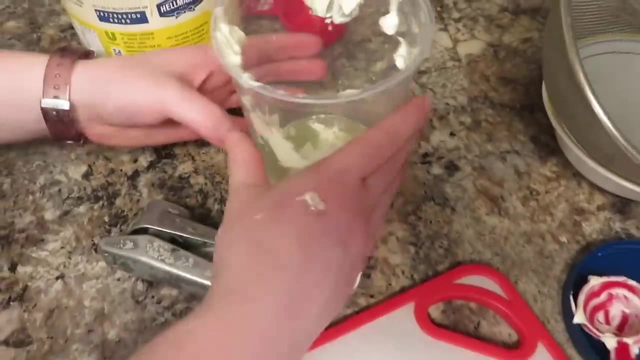 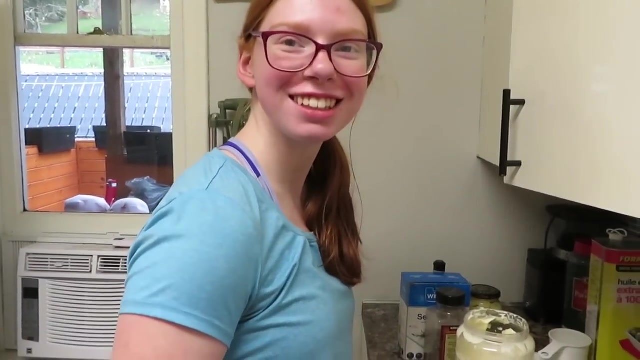 So are you finger painting with the mayonnaise? It's everywhere, Seriously Well, does it look like it's nicely in there? No, I'm just going to push it. Is it all over your hands? It's not that much over my hands. You shouldn't have any on your hands. 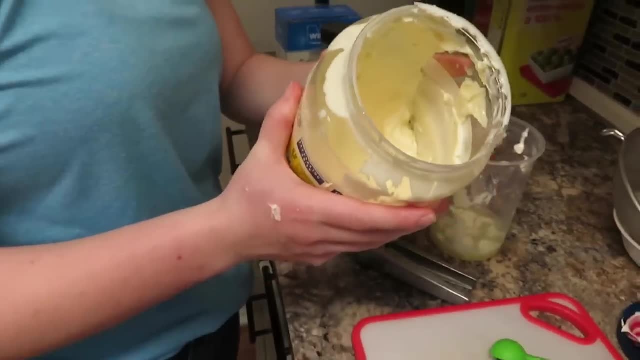 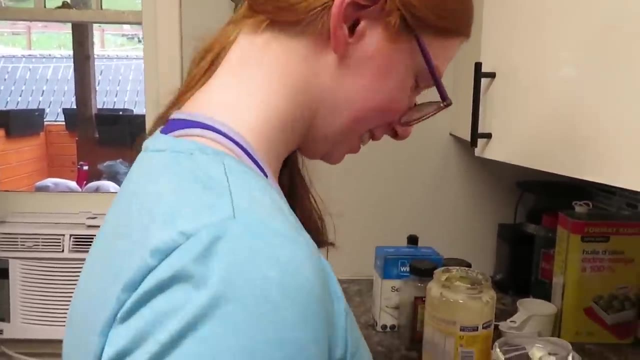 Well, when you're scraping through a dirty hole, I didn't have any problem. Okay, clean up your hands. Okay, clean up your hands. Okay, clean up your hands. Okay, clean up this mayonnaise. Get the lid on, Get it put away. Okay, And let's move on to the next step. 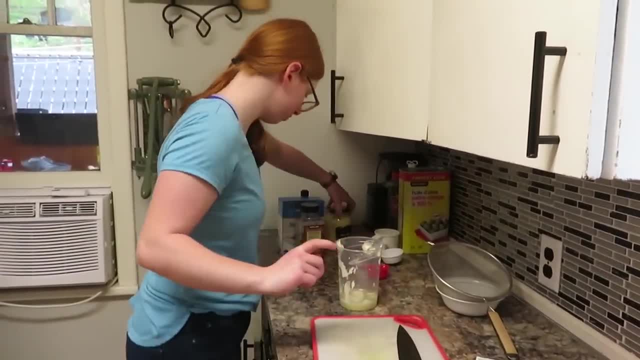 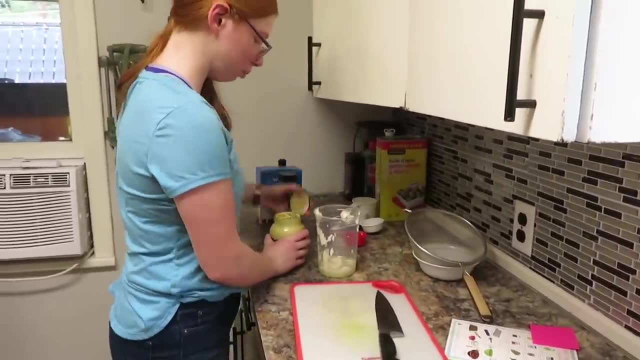 Okay, And now next up is Dijon. How much do you need? One and a half teaspoons, So one teaspoon, You're getting it. Well, it's easy to do with halves, Not at the beginning of our cooking today. Seriously, Seriously. So your salad's ready, Okay, Okay. 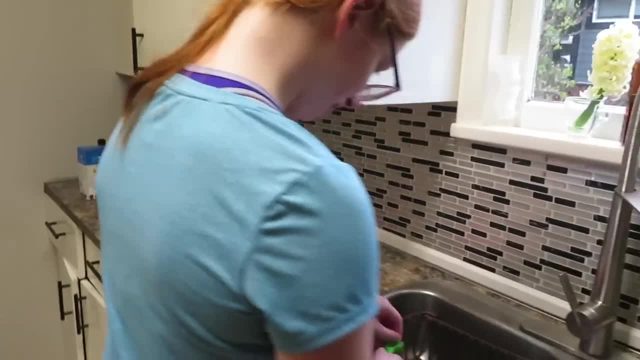 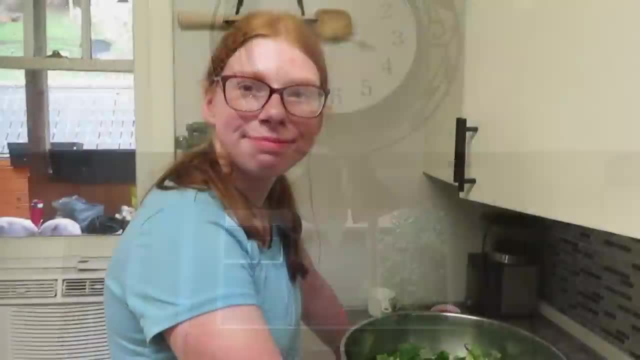 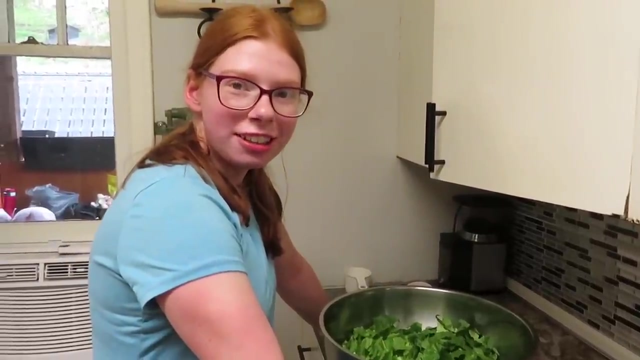 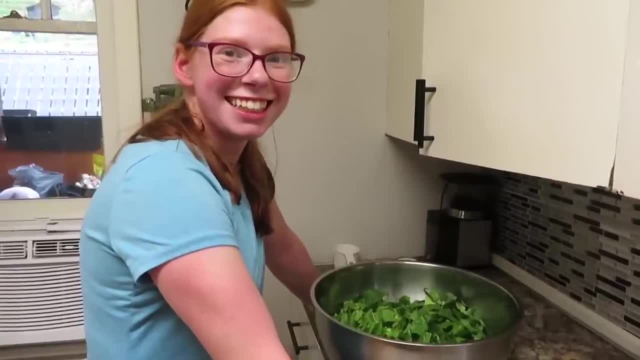 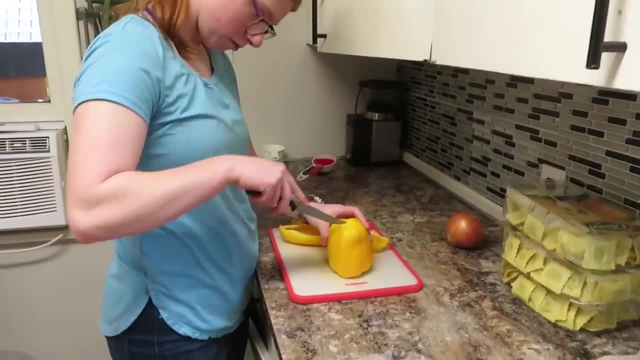 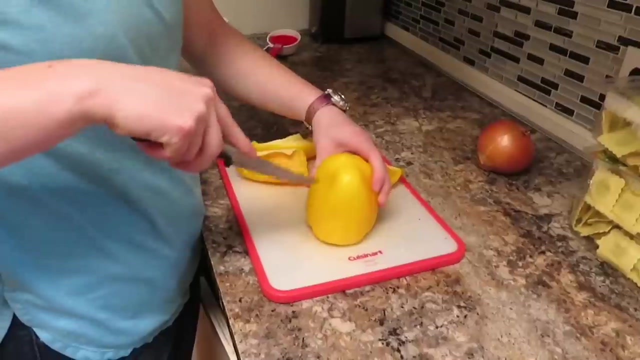 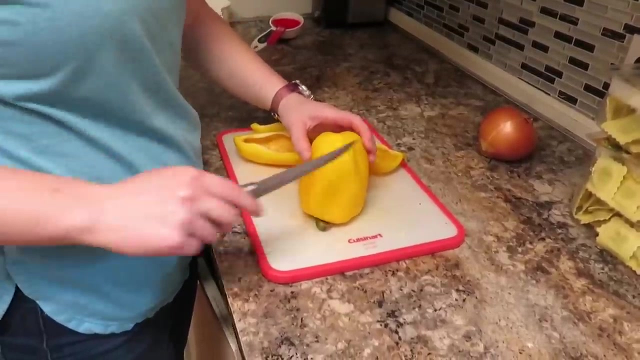 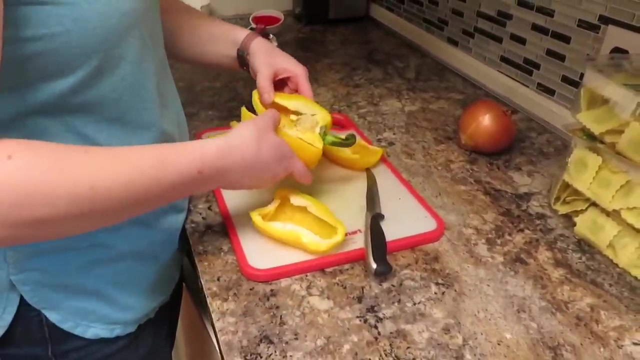 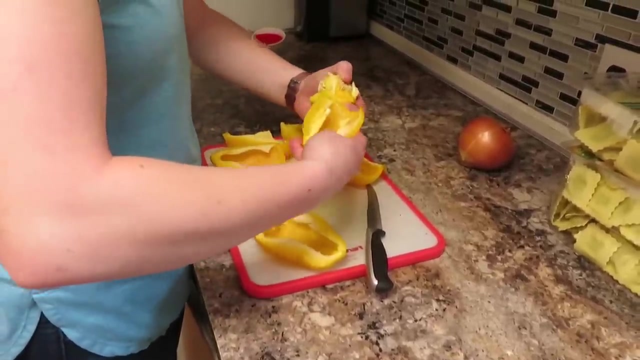 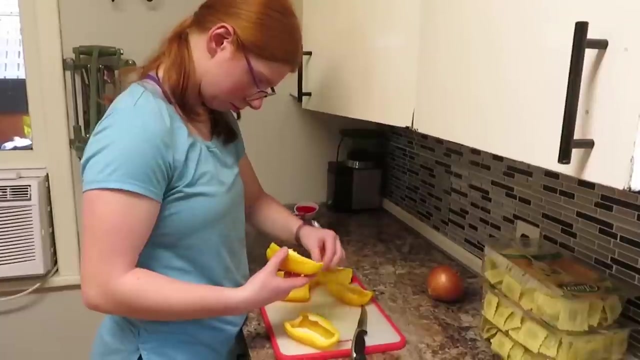 Yeah, You didn't get your big break, But we're back on track. That's good, Okay, So now you have to get the stuff ready for your pasta. Hmm, Mmm, Tasty, How's it going? Good, nice work, thank you. so get the extra bits put into the compost and then we will cut that up. 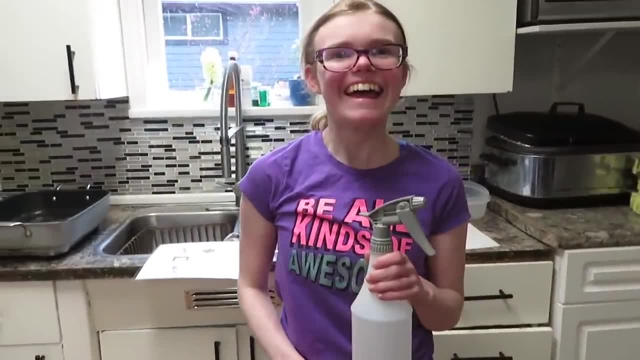 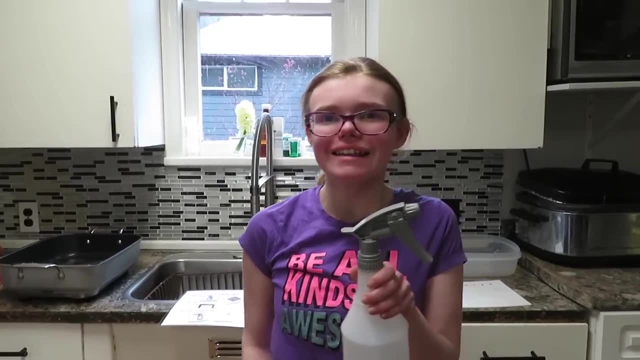 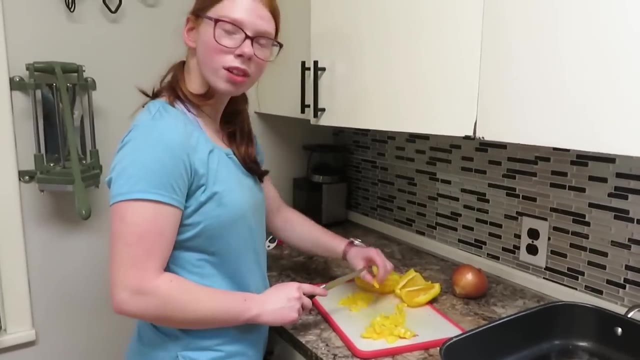 nice and small. so we need you to help Cheyenne- she's doing all this cooking and we need you to set the table. yep, better take your chart. yep, how's the vegetables coming? see how many you can sneak into the sauce. mm-hmm, how long do? 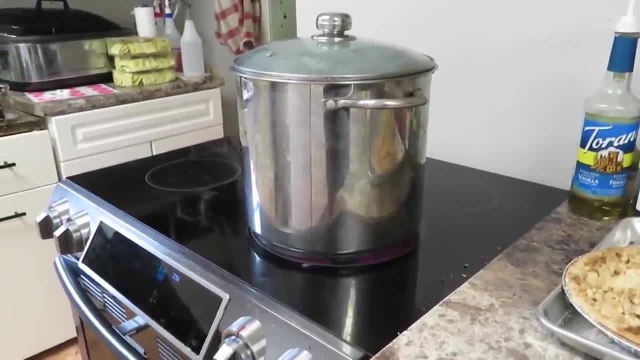 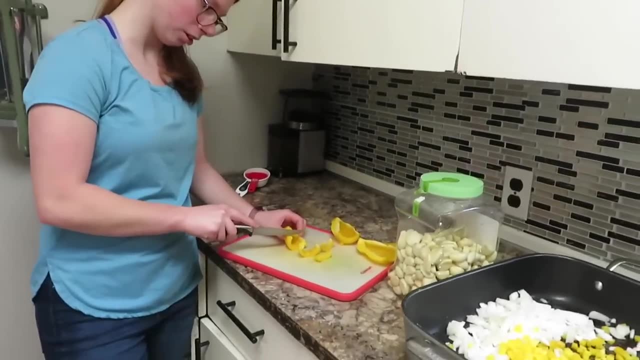 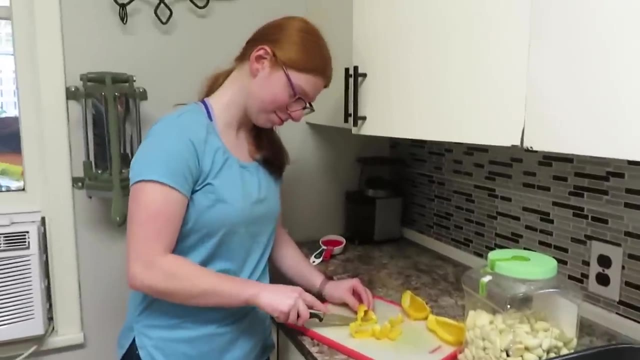 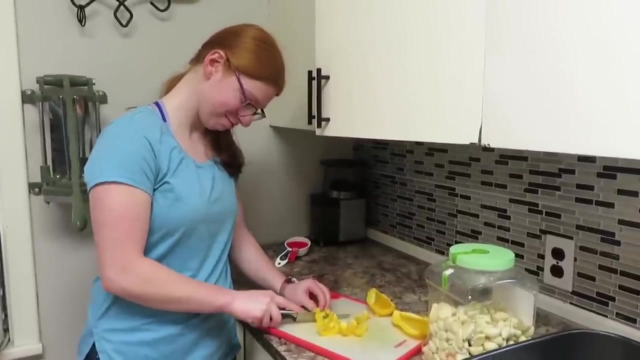 you think it's gonna take for your pork to be ready to be cooked? how long do you think it's gonna take for your pork to be cooked to boil? think that long, okay, and you're getting all your vegetables in here and more garlic, mm-hmm, nice. keep any boyfriends away too. how's it coming? 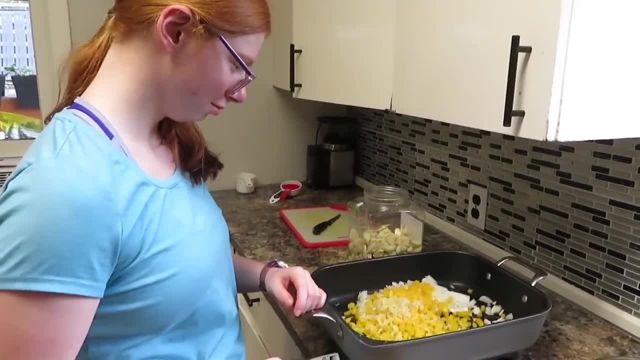 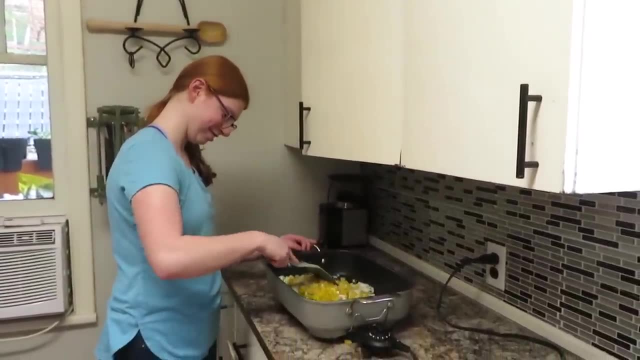 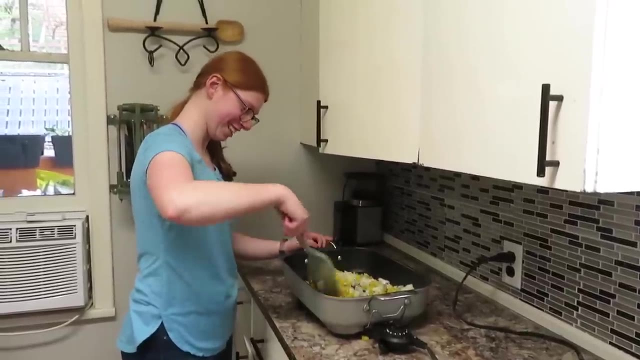 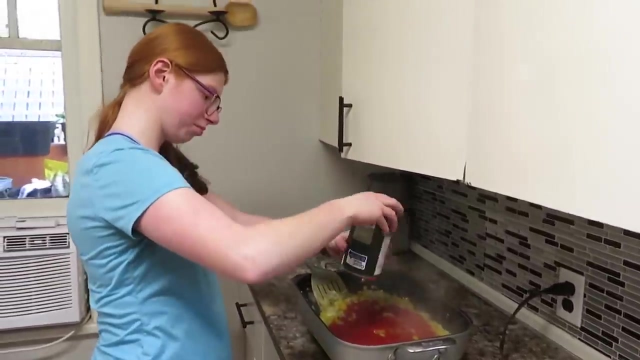 okay, so we need to saute those vegetables up. I'm gonna add some garlic. so how are you holding up? you have been cooking up a storm since 11 o'clock and it's already 420.. feet are tired, your feet are tired. yeah, onions aren't as strong now you don't need to cry, are? 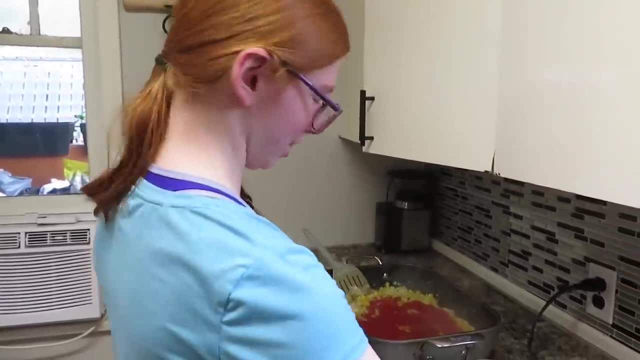 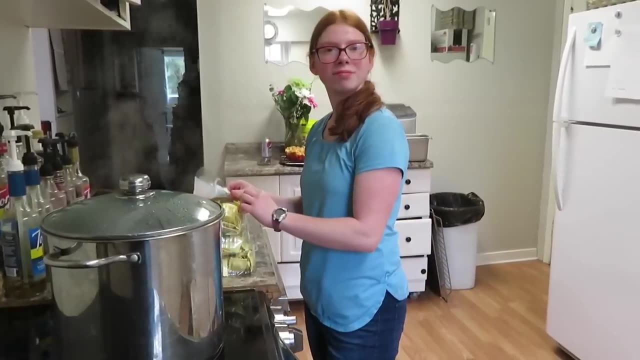 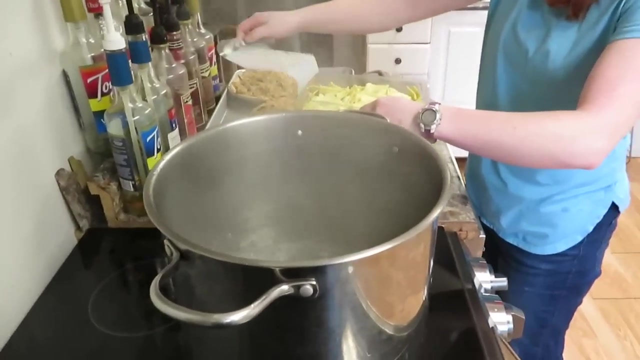 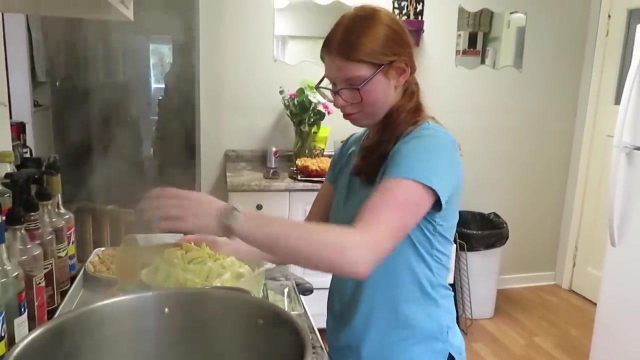 they still bugging you. no, oh, I didn't think they were so strong because they all cooked. You're going to need an oven mitt to get the lid off of this. You dump all the noodles in carefully. Dinner's coming along. Final stretch, Are you? 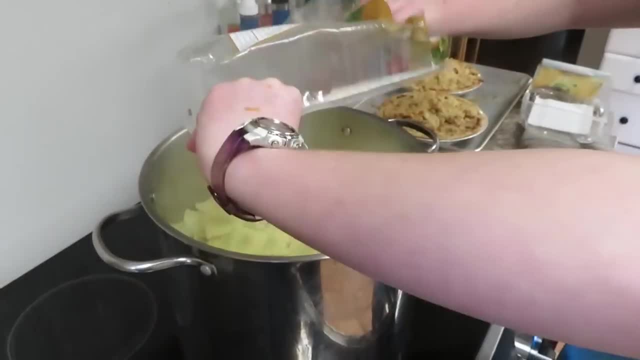 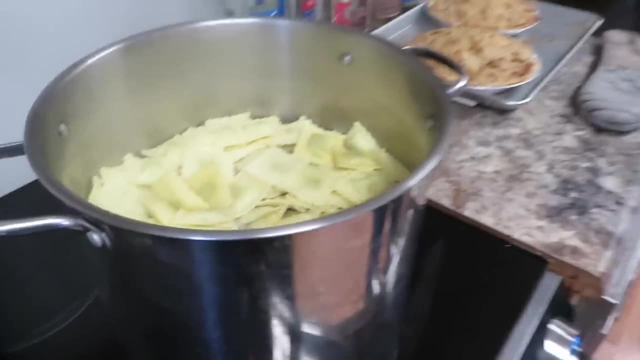 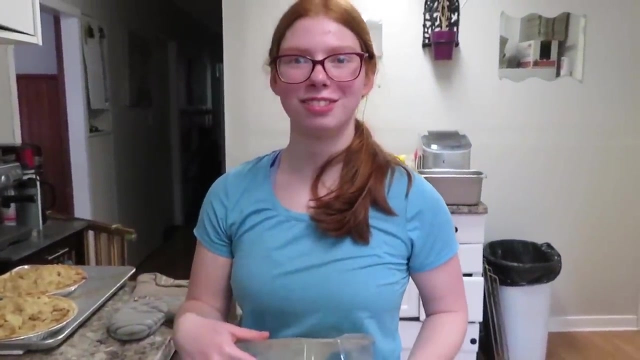 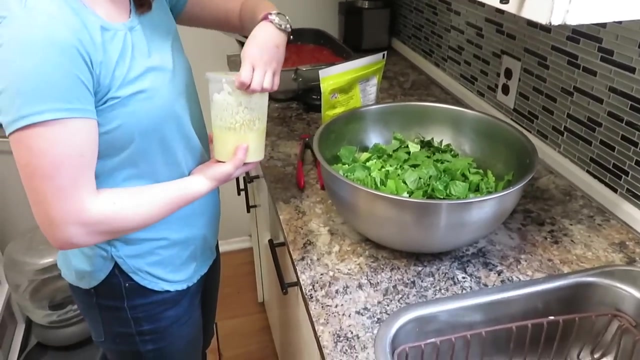 hungry. Yeah, There we go. So those need to come back to the boil, and then they're ready to eat. Mm-hmm, Do you know what you have to do now? What about your salad? Oh yeah, stir those two things together: the dressing and the salad Dressing first. Yes, 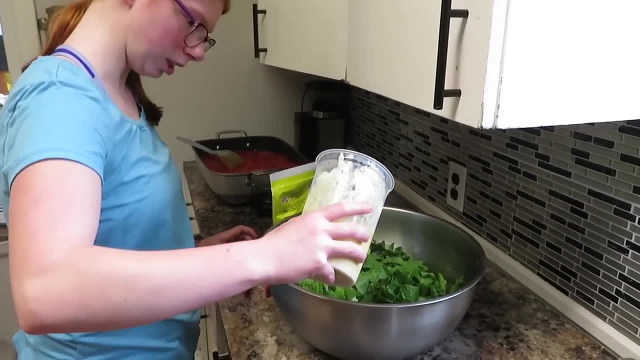 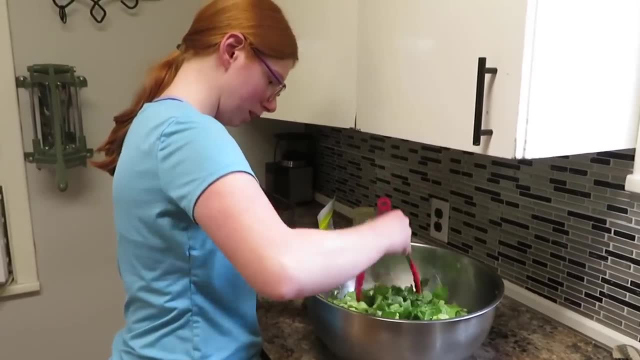 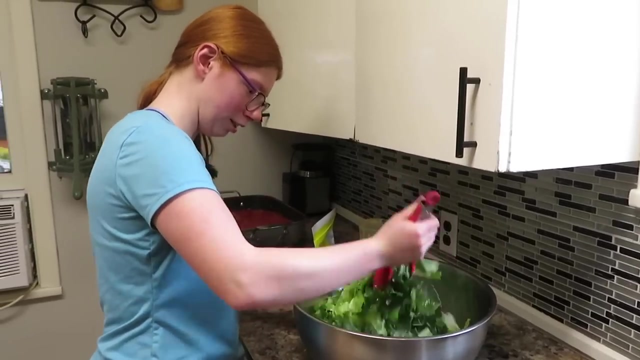 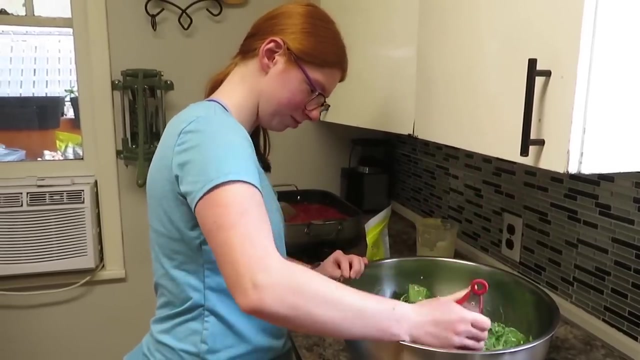 So probably put about half of that on and then start up, so then we can see It's almost time to eat. Mm-hmm, What time is it? 5 o'clock? Yep, it caught up Doing great. You should be really proud of yourself. You made such 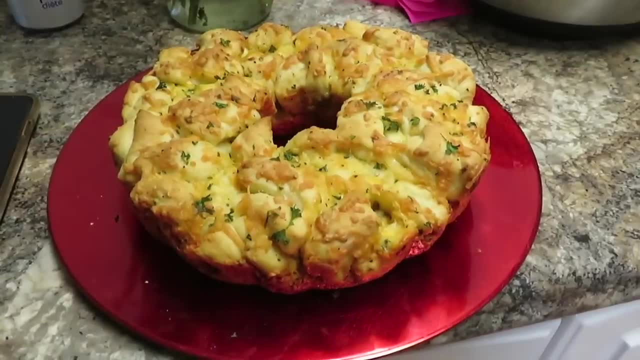 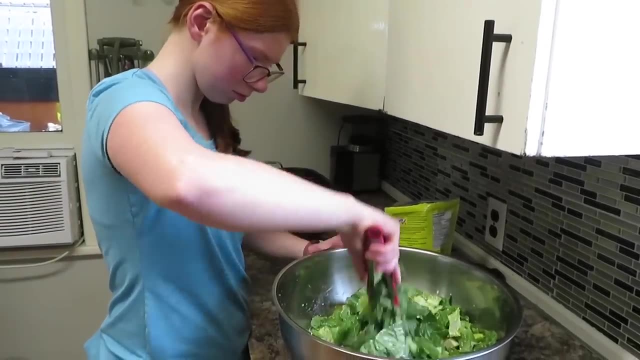 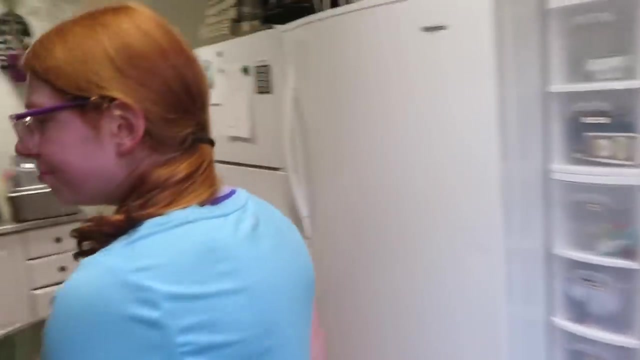 a delicious looking dinner. Mm-hmm, Delicious looking bread. Do you think I need more food times in here? That's probably good. Good, How's it looking? Good? Okay, we can take that to the table. Okay, And I think your noodles are done. Yep, they're foaming.